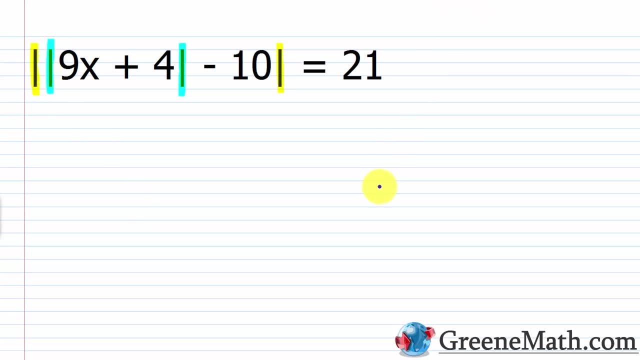 Okay. so the way you kind of attack this problem is you first consider the larger absolute value expression, Okay, the one that surrounds the entire left side of the equation, the one that I highlighted in yellow. So what we're going to do is we're going to set up an OR with this guy. 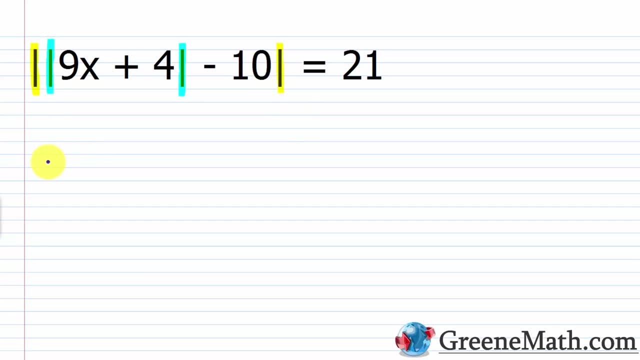 So we're going to drop those absolute value bars. So that would give me the absolute value of 9x plus 4, and then minus 10, and then I'm going to say: this is equal to 21.. Then I'm going to do my OR, So now I'm going to have the absolute value of 9x plus 4.. Okay again. 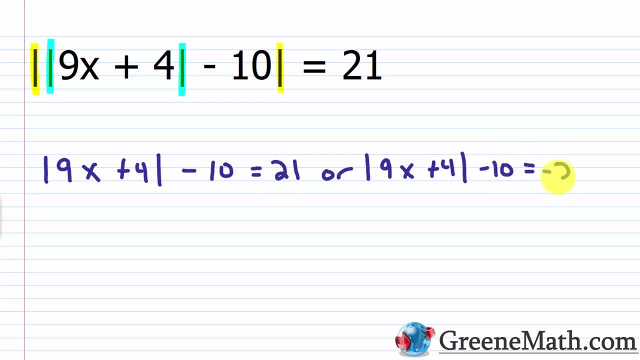 minus 10.. Now it's going to be equal to negative 21.. Okay, so it's the same thought process as what we used in the previous kind of lessons, but we're going to have to do this basically twice. Okay, so it's just extra work, Okay. so for this guy on the left, let me kind of move down just a little bit. 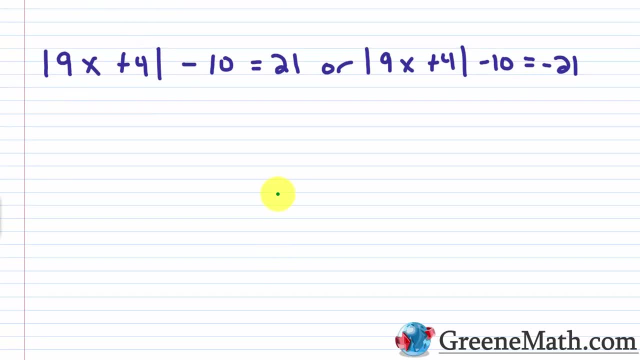 We know how to solve this. This is basically what we've looked at in the past. So let me isolate the absolute value operation. So I'm going to isolate this guy now. So all I'm going to do is I'm going to add 10 to both sides of the equation. I'm going to get that- the absolute value of 9x plus 4. 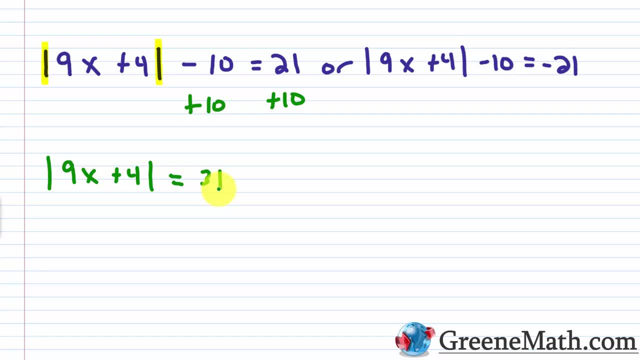 is equal to 21 plus 10 is 31.. Okay, so now all I've got to do is set what's inside of the absolute value operation equal to 31.. Then say: OR, what's inside the absolute value operation is equal to negative of 31.. Okay, so we get: 9x plus 4 is equal to 31, or 9x plus 4 is equal to negative 31.. And 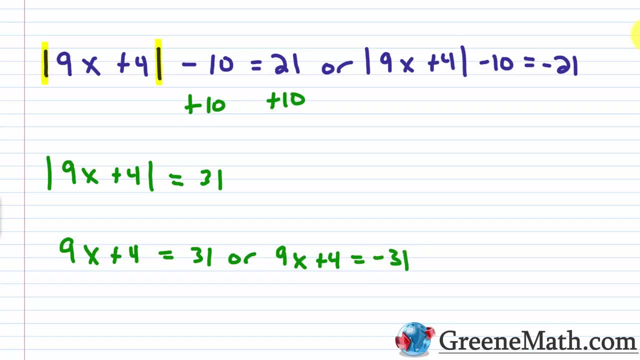 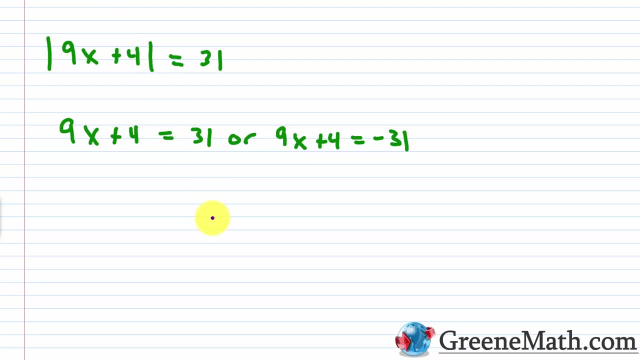 you can see how tedious this becomes. This is just one of those ones where it's not hard once you kind of understand the steps. It just takes a long time, A lot of scratch paper and sometimes that can involve you making some mistakes if you're not really careful. So for this guy on the left I'm 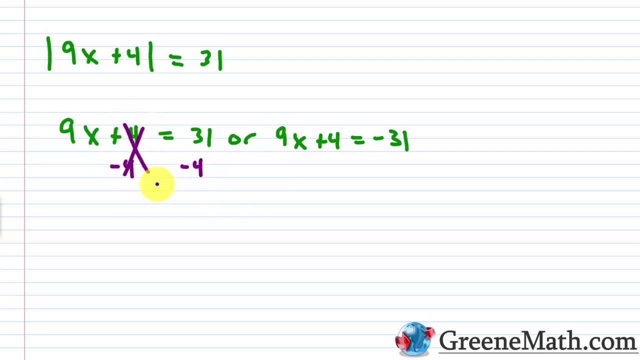 going to subtract 4 away from each side of the equation. This is going to cancel. I'm going to get that 9x is equal to 31 minus 4 is 27.. Okay, so if I divide both sides of the equation by 9, 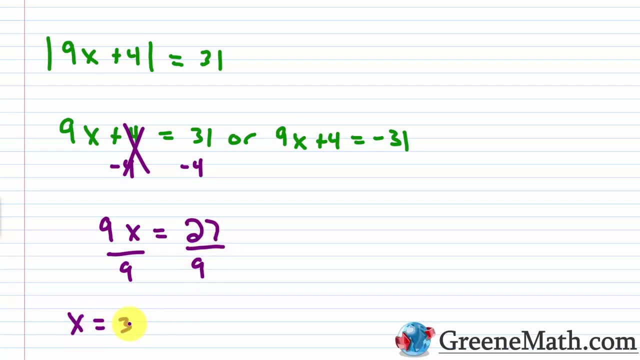 I get one solution, and that's that x is equal to 3.. Okay, so that's one solution Over here. if I subtract 4 away from each side of the equation, this cancels, I'm going to get that 9x is equal to. 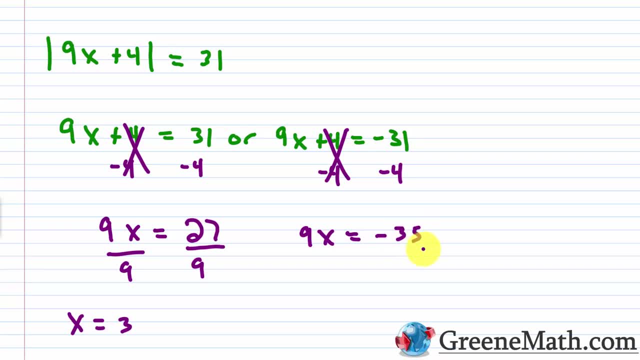 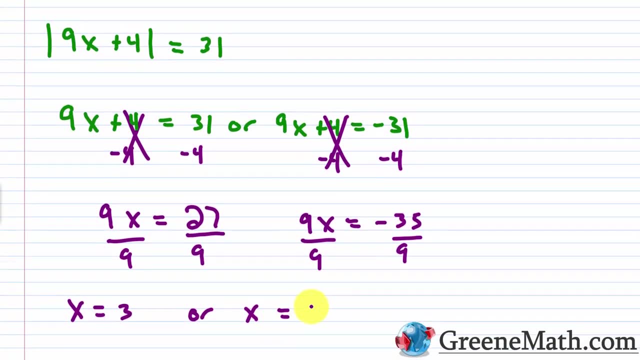 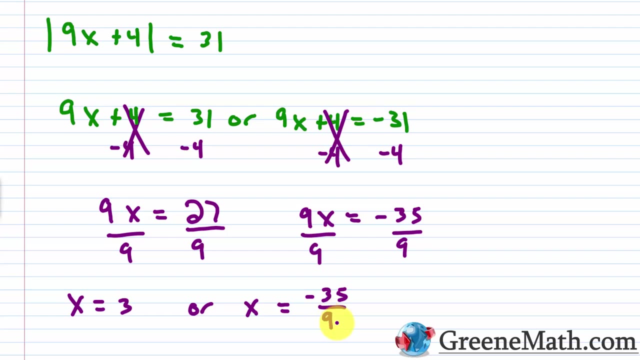 negative 31 minus 4 is negative 35. Again, I'm going to finish this up by dividing both sides by 9. And I'm going to find that x could also be equal to negative 35. okay, So those are two solutions that we have, But we've got to go back up and deal with the 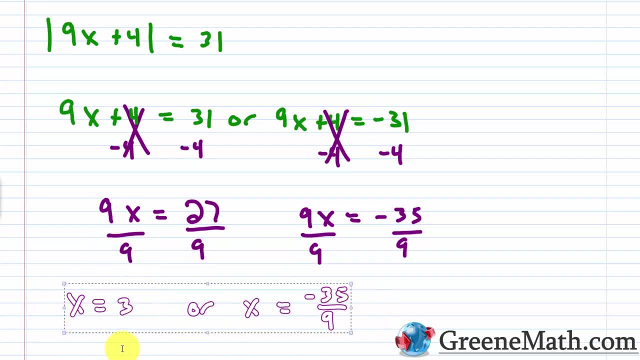 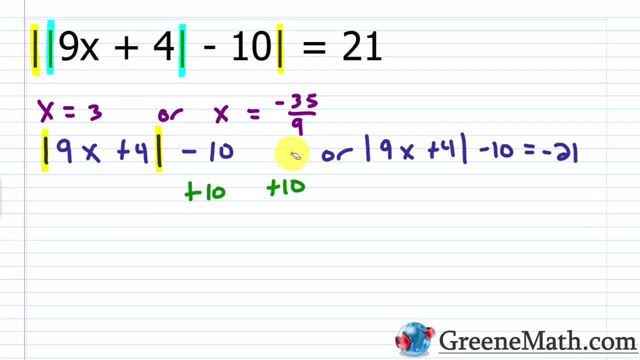 other scenario. So let me just kind of copy this real fast And I'm just going to erase all this work, Okay, and I'm just going to paste that in right here, Right there, Okay, so that's for this guy, right here. So I'm just going to erase all of this. We don't need that anymore And let me. 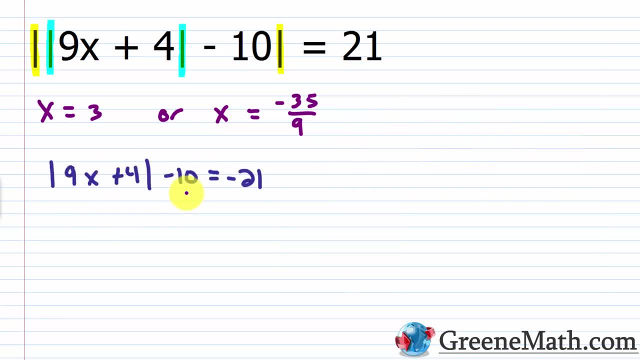 kind of drag this over here And let's work on this guy now. So what I'm going to do is I'm going to add 10 to both sides of the equation to kind of get things started. I'm going to have the absolute. 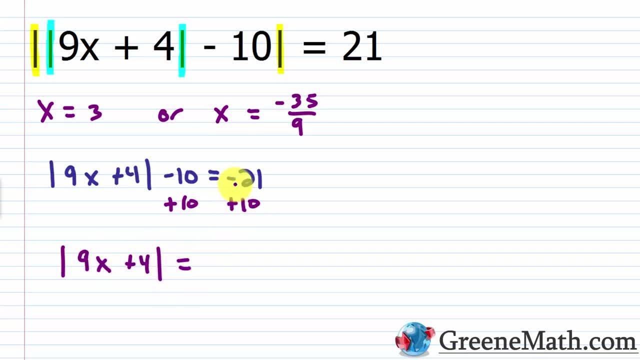 x plus 4 is equal to negative. 21 plus 10 is going to give me negative 11.. Now you'll notice that there's a problem here. We know that if we have the absolute value operation isolated on one side and we have a negative value on the other side, there's no solution. Okay again, if I take the 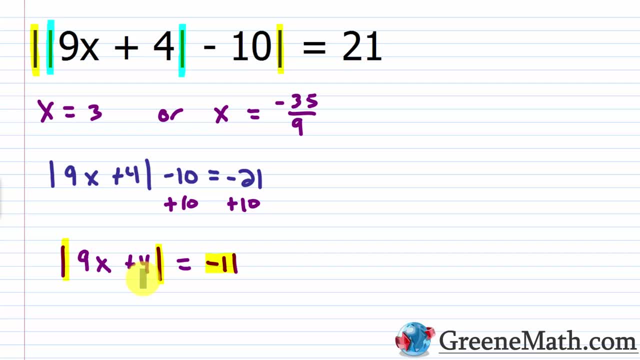 absolute value of a negative number, it becomes positive. If I take the absolute value of zero, I get zero. If I take the absolute value of a positive, it stays positive. So there's nothing I can do about that. So what I'm going to do is I'm going to take the absolute value of 9 and then 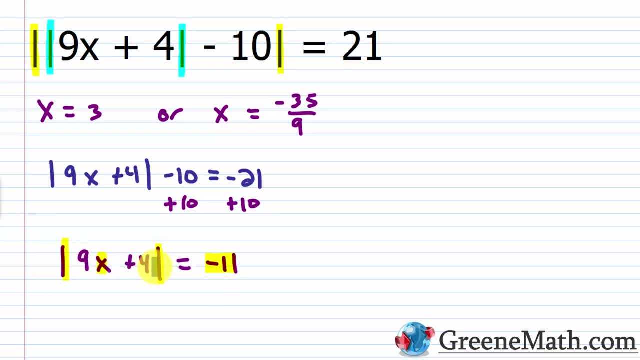 take that and add to 4, and take the absolute value and get a negative 11. Okay, it's not going to happen because again, the absolute value operation is going to give you a non-negative result, And so this guy could never be equal to negative 11.. So for this part we would say there's no solution. 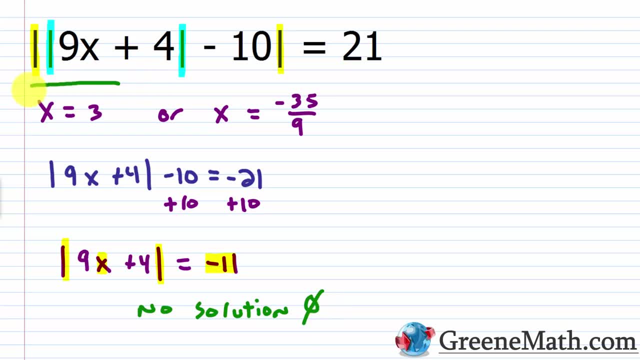 Okay, there's no solution. Okay, but for the equation as a whole, we found one part had a solution, So this is going to be the solution for the whole thing. This guy- you can just throw it away, Right type of answer. Okay, so for this guy as a whole, the solution is going to be x could be 3 or x could. 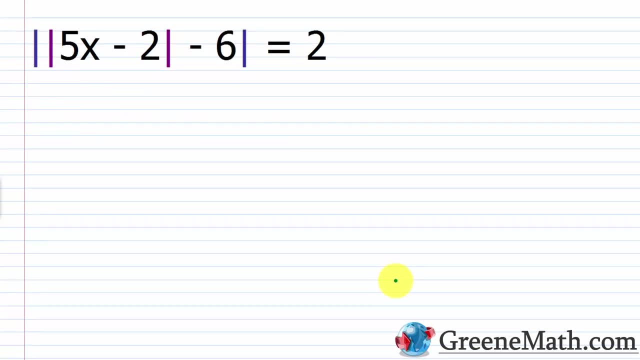 be negative 35 ninths. All right, let's take a look at another one of these, and then we'll move on and talk about another type of problem that you'll probably encounter. So we have the absolute value of, and then inside of that, you have the absolute value of 5x minus 2 and then minus 6.. This whole. 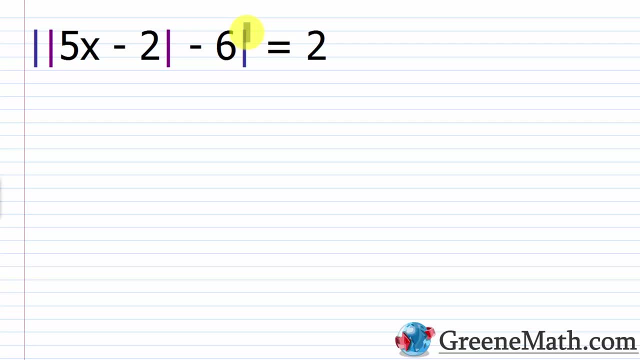 thing is equal to 2.. So, again, I'm going to start with the outside absolute value operation, And what I'm going to do is I'm going to set up two scenarios. I'm going to say that the absolute value of 5x minus 2 minus 6 is equal to 2.. Then, or I'm going 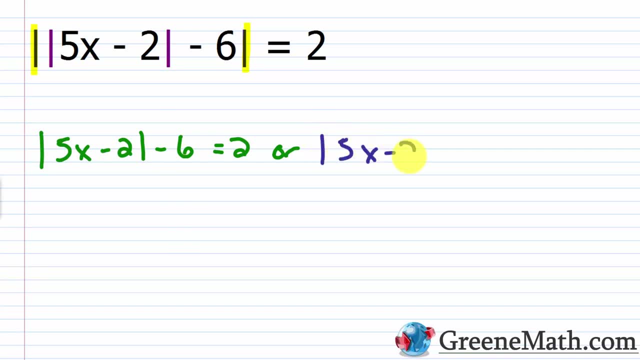 to also say that the absolute value of 5x minus 2 minus 6 is equal to what It's equal to the negative of 2.. Okay, so just split it up into two cases, and then we're just going to start working. 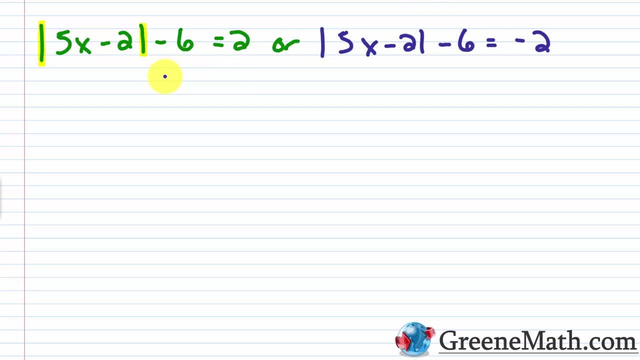 So over here I know I want to isolate the absolute value operation, So I'm going to do that by adding 6 to both sides of the equation. So I'm going to get that the absolute value of 5x minus 2 is equal to 2 plus 6 is going to be 8.. Okay, so this splits up into two more cases. 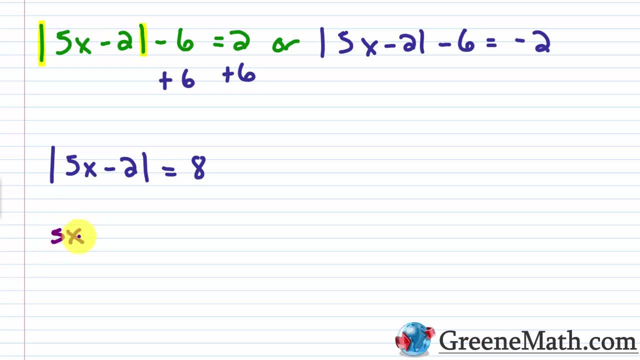 right. So we can say that 5x minus 2, this expression inside the absolute value bars- is equal to 8, or 5x minus 2 is equal to negative 8.. Okay so let's solve those real quick, we'll. 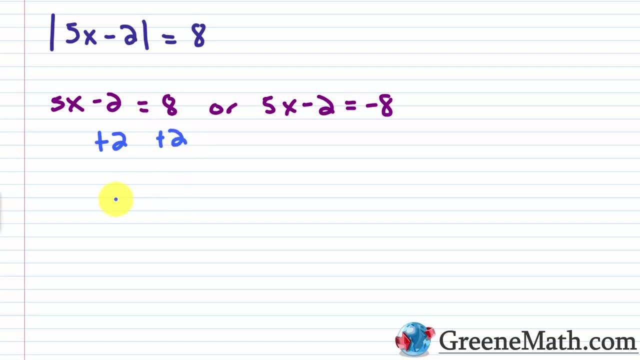 come back up. So let me go ahead and add 2 to both sides of the equation. We're going to have that. 5x sides of the equation by five. we're going to get that x is equal to two. Okay, so that's one. 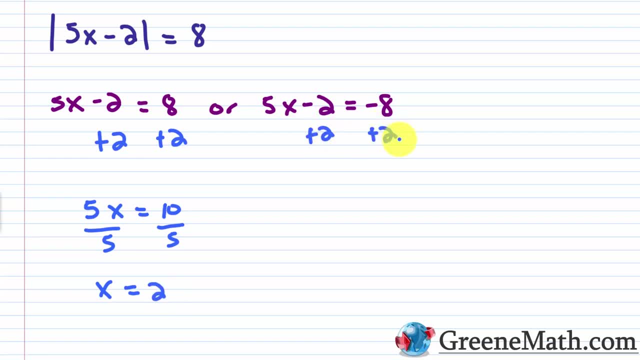 solution Over here. let me add two to both sides of the equation And I'm going to get that five. x is equal to negative six. divide both sides by five and I'm going to get that x is equal to negative six fifths. Okay, so we have two solutions. we've got x is two or x is negative six fifths. 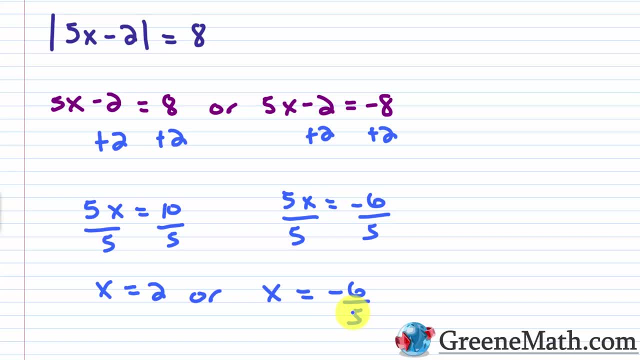 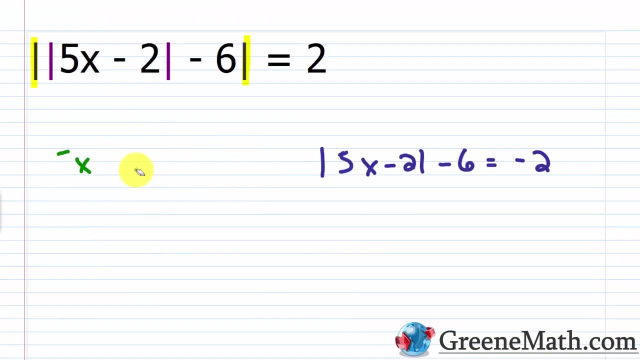 So let's work on the other side and see about getting some more solutions. Okay, so let me just copy these And I'm going to erase all this work. we don't need it anymore. Alright, so I'm just going to erase this part right here And let me just drag this other one over here, because we 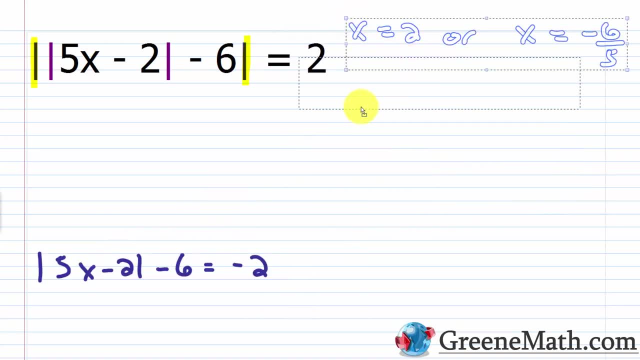 need to work with this And I'm just going to paste these solutions in. this is what we have so far And I'm just going to erase this and put a little comma. So x equals two, and I'll put comma negative six fifths. Okay, let's take a look at this kind of second case. So again, we want to. 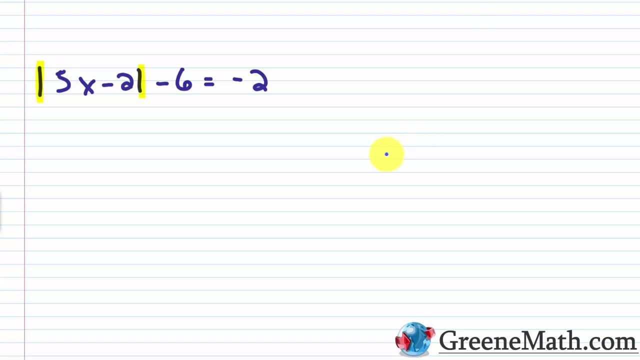 isolate the absolute value operation, And what we're going to do is just add, say x to both sides of the equation, And so this guy is going to cancel. we would have that the absolute value of five x minus two is equal to what negative two plus six is positive four. So in the other 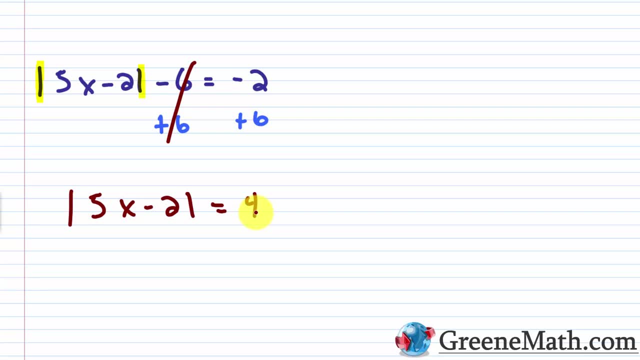 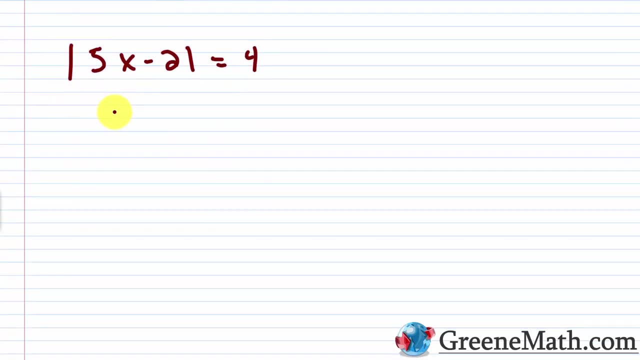 example, we saw that in our kind of second case we had something with no solution. In this example we don't have that, so we can keep going. So what we're going to do is again set this up into two more cases. So five x minus two, the expression inside the absolute value bars could be equal to: 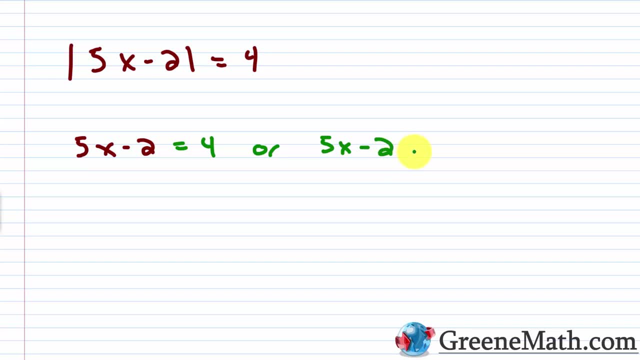 four or five x minus two could be equal to negative four. Okay, so we're just going to solve those two scenarios. So let me add two to both sides of the equation here. I'm going to get that five. x is equal to six. divide both sides by five, we're going to get x is equal to six fifths. Okay. 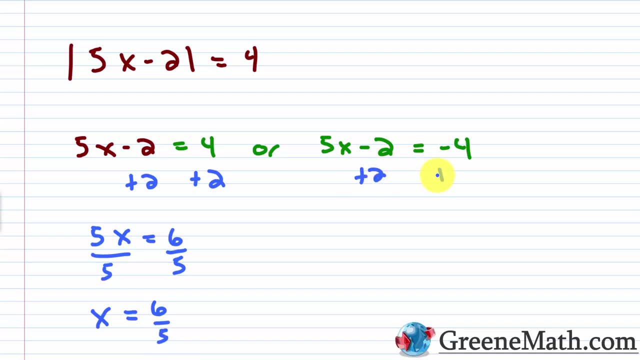 so that's the solution Over here. I'm going to add two to both sides of the equation. I'm going to get that five x is equal to negative two. we're going to divide both sides by five, so I'll put or. here x could also be equal to negative two fifths Okay. so we're going to have. 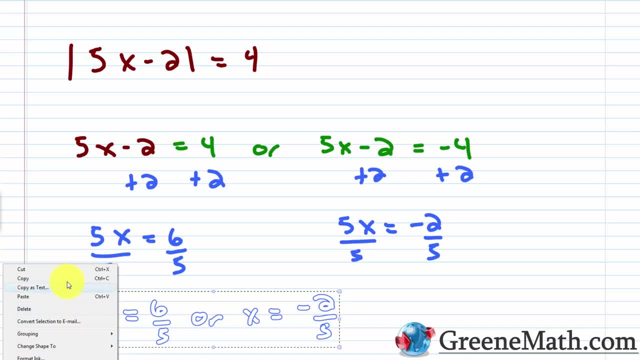 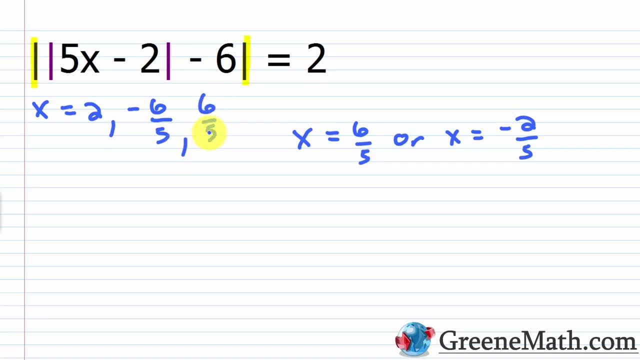 a total of four solutions. Let me kind of copy this And I'll erase everything. Okay, so we have six fifths and negative two fifths. So let me put comma six fifths and comma negative two fifths. Okay, so those are our four solutions. I'm not going to check them in the interest of time. 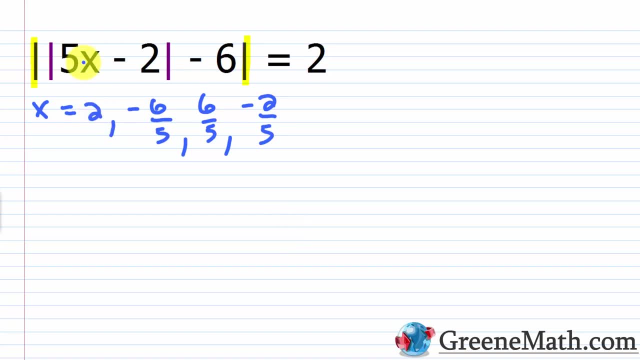 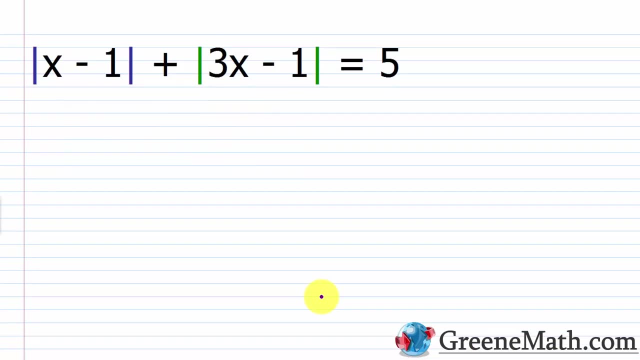 But you can plug each one in for x And you see that you get a true statement in every case, right? So x is two negative, six fifths, six fifths or negative two fifths, Alright, so now let's move on and look at 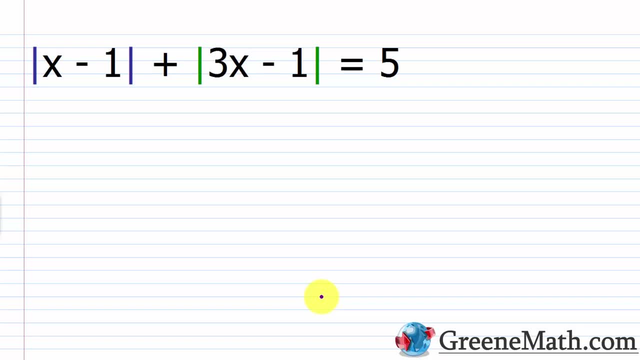 something that's even more tedious. So we've previously seen examples where two absolute value operations were directly set equal to each other. Okay, So for that scenario it's very easy to solve. But what happens when we have an equation with two absolute value operations? 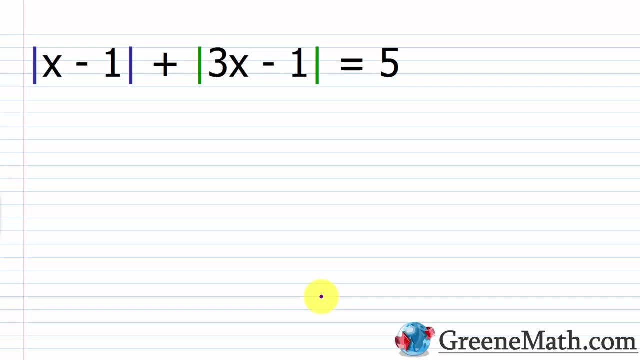 and then kind of an extra or a loose number. Okay, so this is a very common scenario that you'll come across. So something like the absolute value of x minus one, then plus the absolute value of x minus one, and this is equal to five. Okay, So in this case we can't directly set the two. 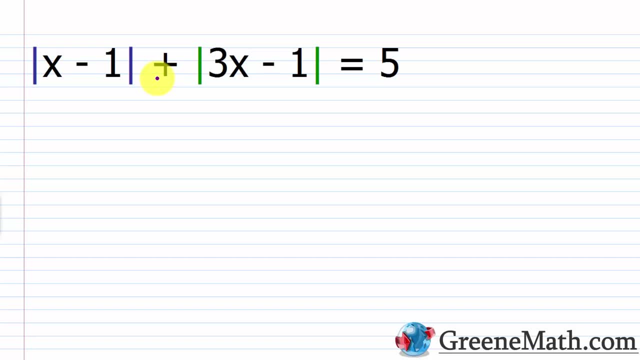 absolute value operations equal to each other. Okay, so we can't use that method, So we have to kind of turn to a more advanced approach, or, you could say, a more tedious approach. Now there's other ways to do this than what I'm going to show you, And I'll explain that when I get done with 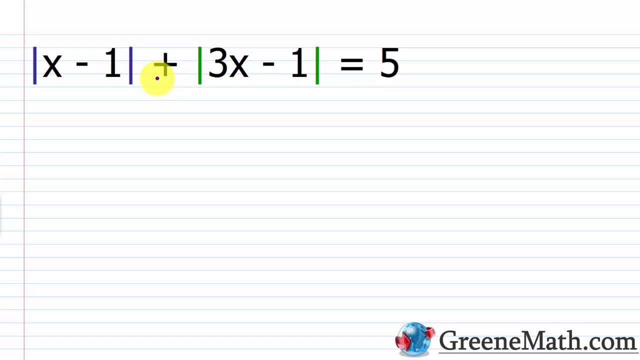 this method. So what we're going to do is we're going to think about the expressions that are inside of the absolute value operations. So you've got two of those, Okay. So what we want to do is we're going to look at the expression x minus one plus one, Okay. So what's going to happen is: 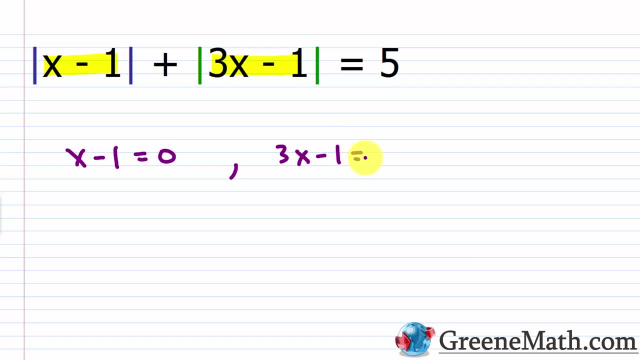 we're going to sum up all the equations together, okay, so we're going to start with the positive and the negative. So where do those two expressions equal to zero? Okay? so where is the expression x minus one equal to zero? And where is the expression three x minus one equal to zero? Okay? 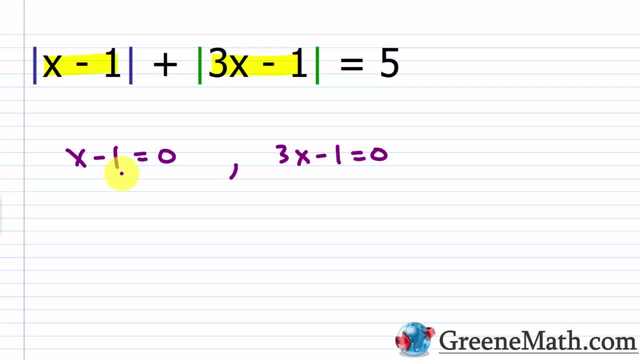 because those represent basically our turning points- is where the sign is going to change from positive to negative or from negative to positive. Okay, this can only happen at a value of zero. So for this one- I'm just going to solve- I'm going to add one to both sides of the equation. So I'm going to have that x is equal to one. Okay, for this one, I'm going to add one to both sides of the equation. So if I'm going 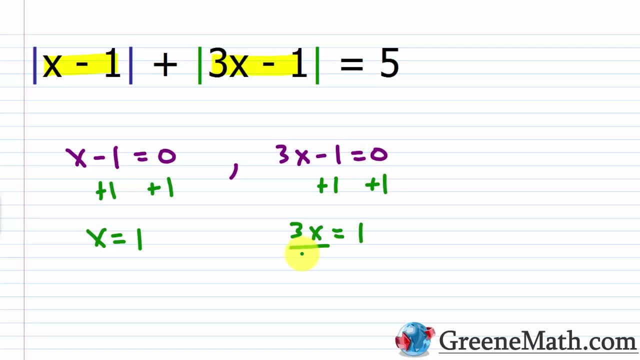 equation, I'm going to get that 3x is equal to 1. I'm going to divide both sides of the equation by 3 and I'm going to say that x is equal to 1. third, so this value here of 1 is what makes this. 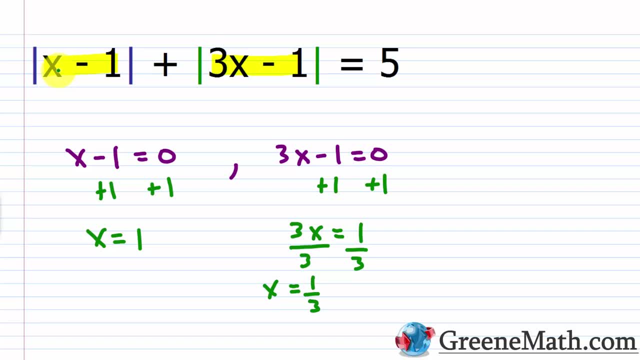 expression here equal to 0, right? if I plugged in a 1 there, 1 minus 1 would be 0. okay, this value of 1. third is what makes this expression equal to 0, 3 times the third is 1. 1 minus 1 is 0, so we can. 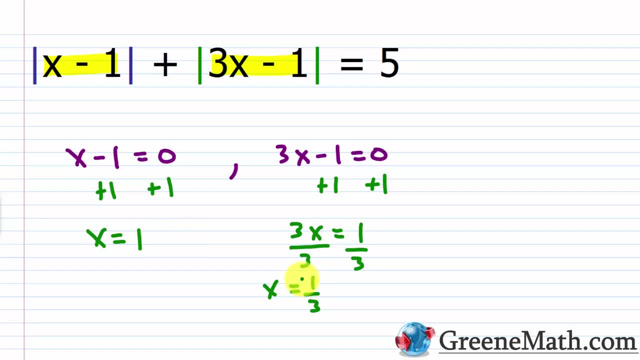 see that. so we're going to use these two values to kind of split the number line up into intervals. so let me go down here real quick to a little table. so this is a good way to kind of organize the information. so one interval would be anything from negative infinity up to, but not including, 1. 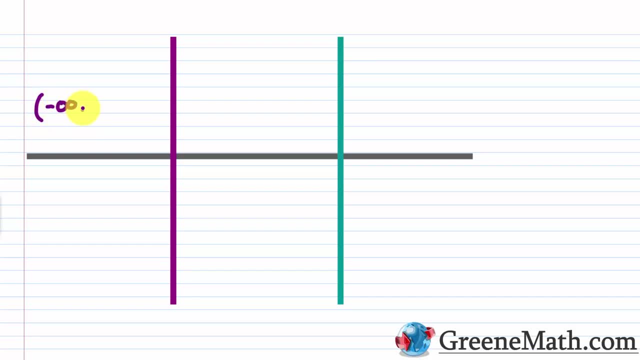 third, so this interval here. so we have negative infinity and we have 1 third and again, neither of those is going to be included here. then the next one: if we go back again, the values were 1 third and 1, so I want to think about between 1 third and 1, what's going to happen? so what happens? 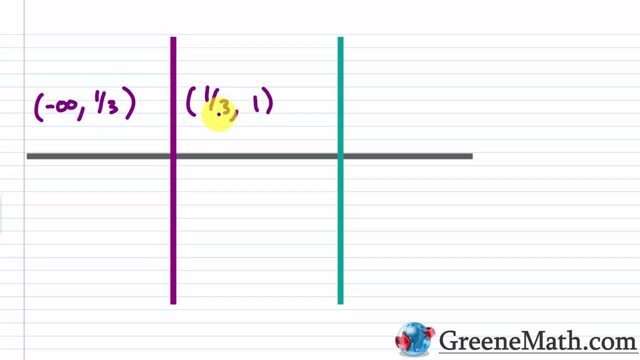 between 1 and 1, so I'm going to go back and I'm going to go back, and I'm going to go back, and I'm 1, 3rd and 1.. Okay, neither of those is going to be included. And then my last interval would be: 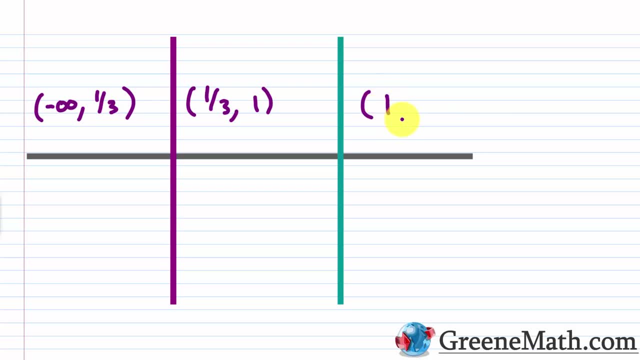 anything greater than 1.. So I'll put a 1 next to a parenthesis and then comma: infinity. Okay, so that interval there. So what we're doing here, in case you're confused, we're thinking about the value of the expression in each interval. Okay, so if it's negative, we're going to replace. 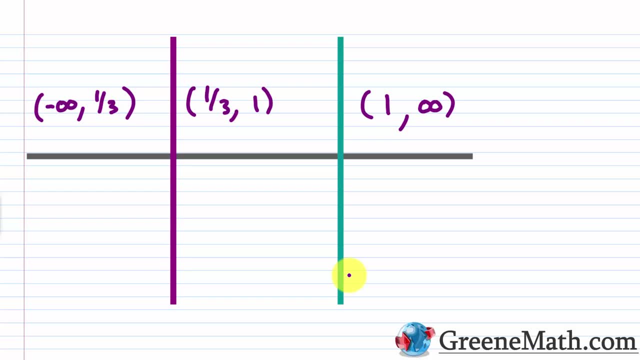 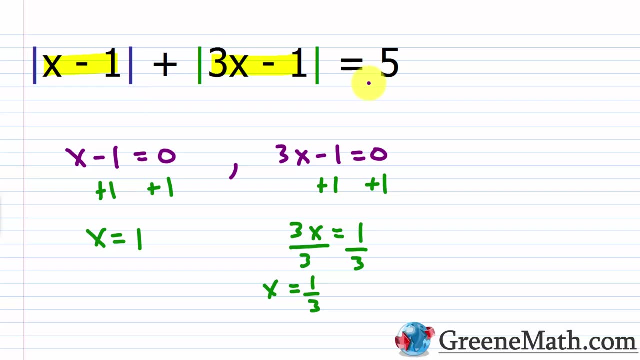 the expression with the opposite, And if it's positive, we just replace it with the expression itself. Okay, So if I go back up again, this guy right here, I'm just going to copy this down here. So we have the absolute value of x minus one, then plus the absolute value of three x minus. 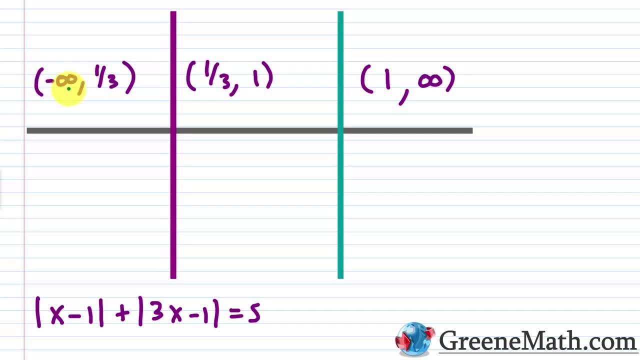 one, this is equal to five. So when we think about this interval- anything that's less than 1- 3rd- we know that both of these guys would be negative. Okay, because this guy right here is zero when x is equal to one, And this guy right here is zero when x is 1- 3rd. 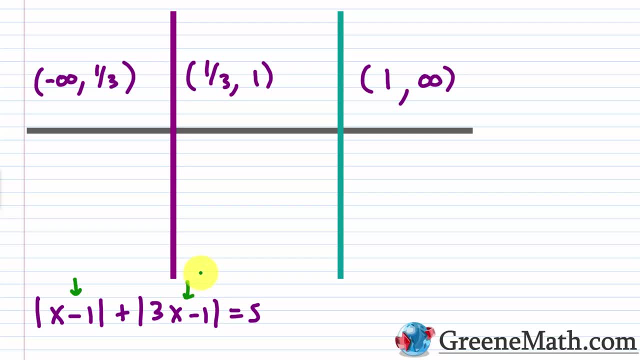 So. So if it's less than one-third, both of those guys would be negative, and so you would take each expression, okay, each expression, and you would make it into its negative or its opposite, okay. So in other words, this guy would be negative of x minus 1, that quantity. 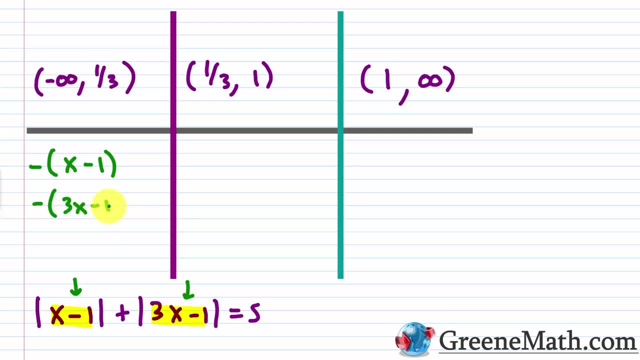 This guy would be the negative of. you have 3x minus 1, that quantity. okay, So that's the expressions. We're going to be dropping the absolute value bars in each case and we're going to be replacing those with these kind of expressions we're setting up here. 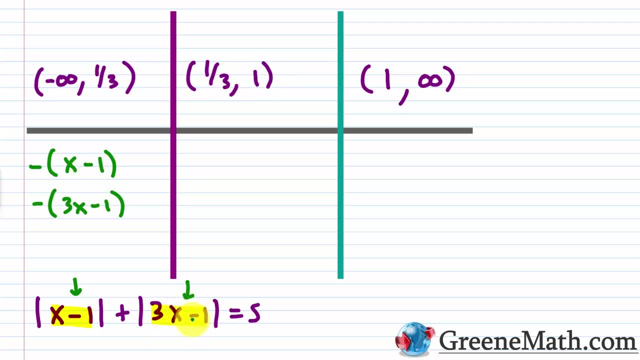 Now between these two numbers, one-third and one. remember, this guy is made zero by one-third, So anything larger than one-third means that this guy is going to be positive. So I can replace this one with the just expression itself: so 3x minus 1.. 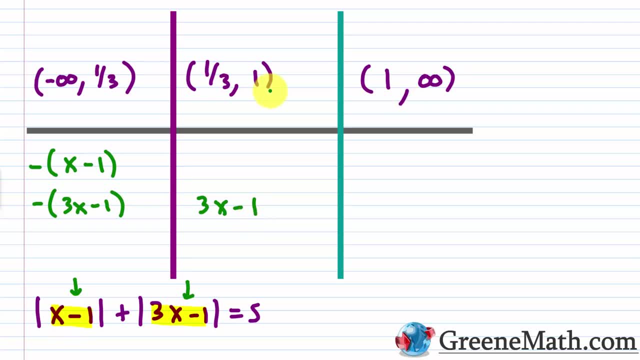 Then for this guy right here again, one is what makes it zero. so anything that's less than one is going to result in this being negative. so this is negative of the quantity x minus 1.. Then in this scenario here, where we're larger than one, we're going to replace this one. 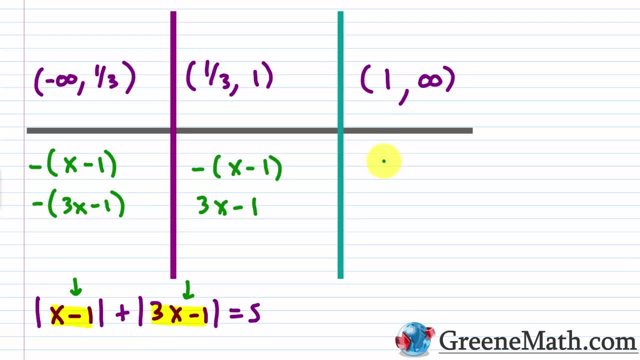 with the expression itself. so 3x minus 1.. Then for this guy right here, again, one is what makes it zero, so anything that's less than one. both of these guys are going to be positive, so I can say this is x minus. 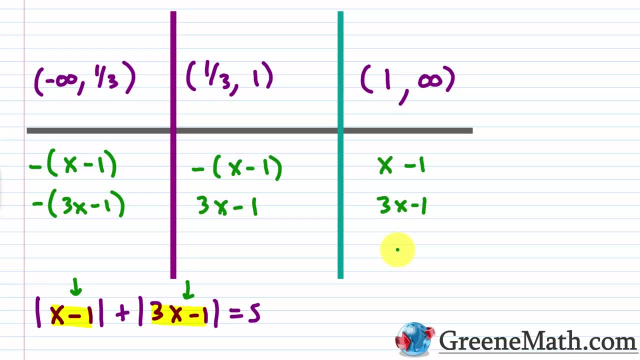 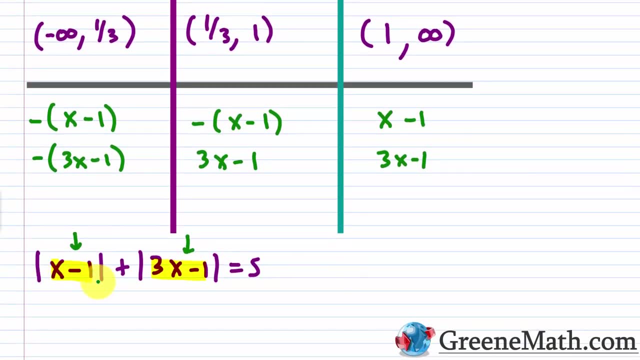 1, and this is 3x minus 1,. okay, So what I'm doing here is I'm going to go through- let me kind of scroll down a little bit- and I'm going to basically replace my absolute value expression in each case with: 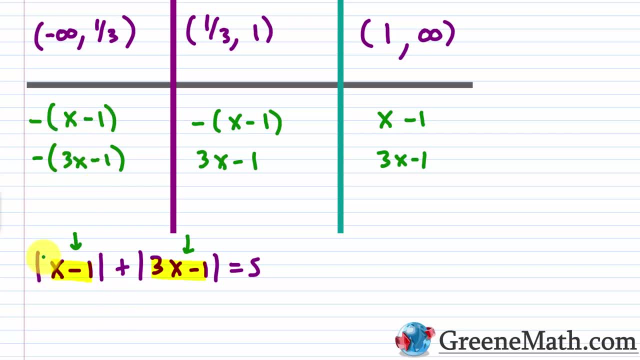 what I came up with for the interval. So for this first interval, instead of having the absolute value of x minus 1, because this guy is negative, I'm going to say it's negative of x minus 1, then we would have plus you'd. 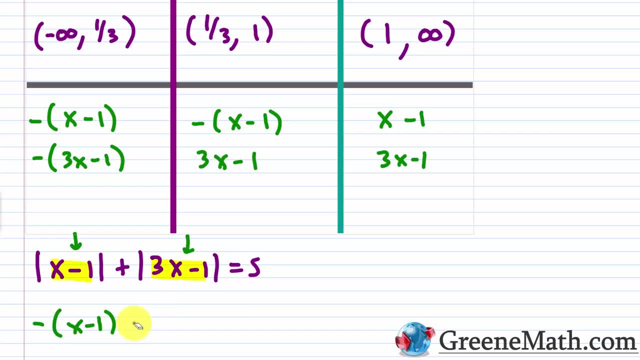 have the negative of this guy as well. so you could put plus negative or you could just put minus, doesn't matter. so minus, you have the quantity 3x minus 1, and this is equal to 5, okay. 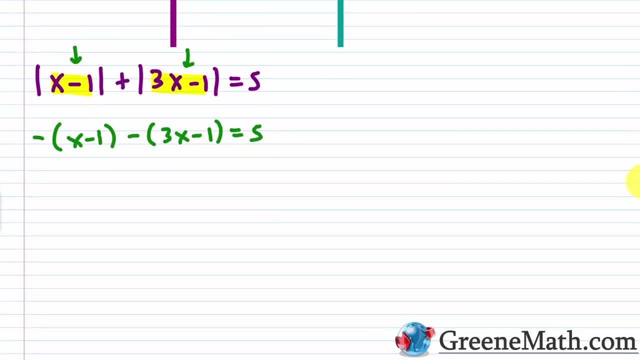 So let's scroll down and solve this and then we'll come back up. we just want to make sure we have enough room, So I'm going to distribute the negative to each part here. so this would be negative x plus 1,. distribute the negative, so negative 3x plus 1, and this equals 5.. 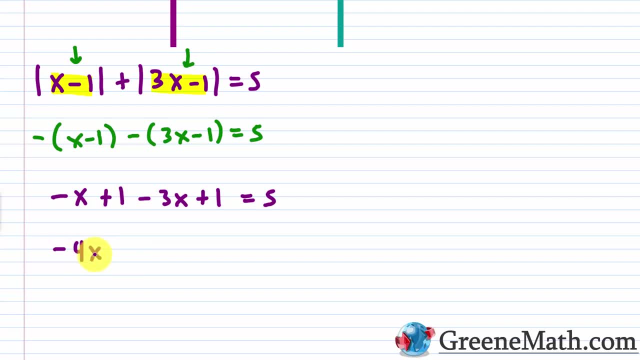 So negative x minus 3x would give me negative 4x. 1 plus 1 is 2, so plus 2.. This equals 5, and then what I'm going to do here is I'm going to subtract 2 away from. 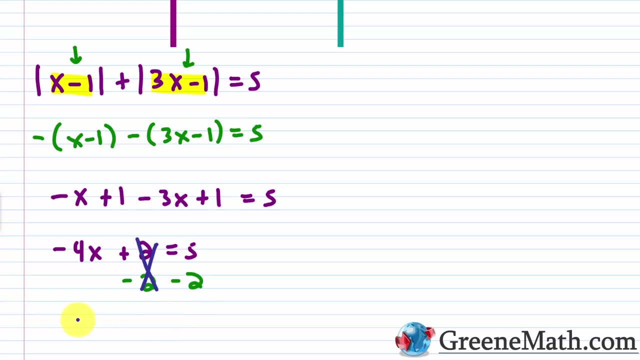 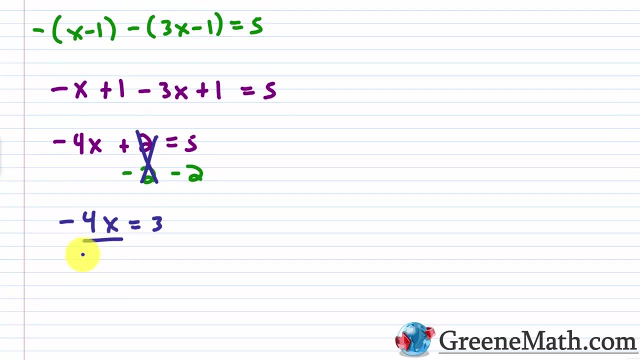 each side of the equation and we're going to find that this is going to cancel. we're going to have that negative 4x is equal to 3, we're going to divide both sides of the equation by negative 4, so divide this by negative 4, and this by negative 4, we're. 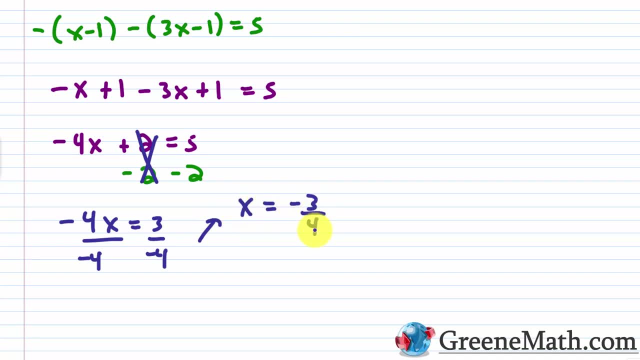 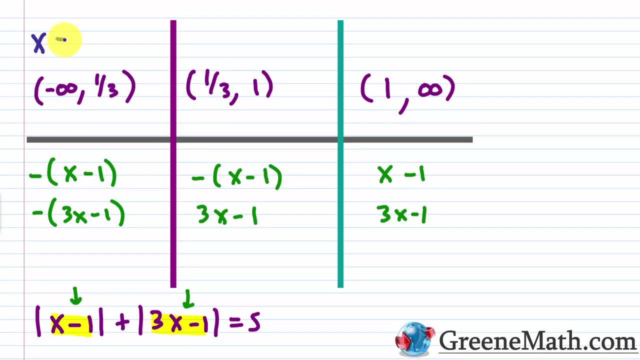 going to get that x is equal to negative 3 4ths. okay, So I want to erase everything and I want to show you what we do here. so let me erase all this. So the solution we found in this interval is that x is equal to negative 3 4ths. 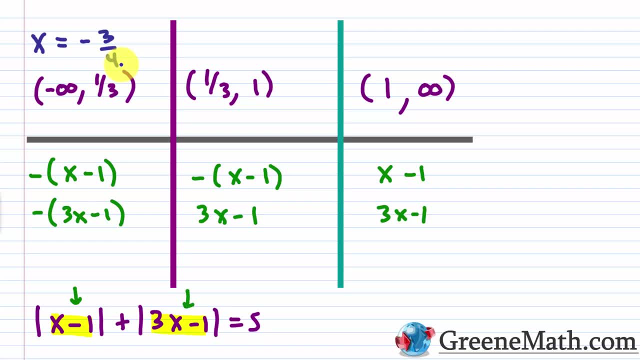 Now, what you end up doing in this process is: if your solution lies in the interval, you accept it. If it lies outside of your interval, then you're going to reject it, Since negative 3- 4ths is in this interval, right from negative infinity up to, but not. 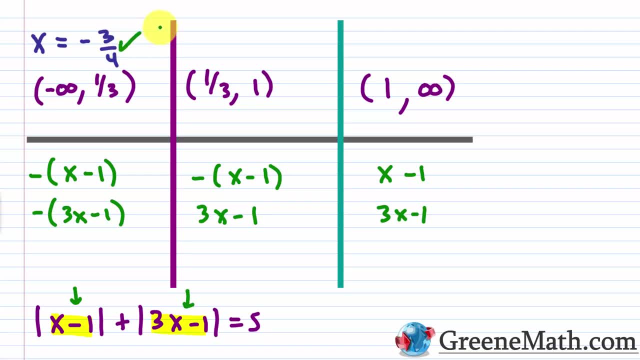 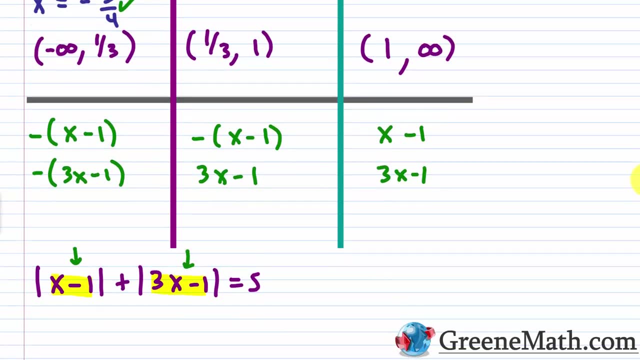 including 1- 3rd. we can accept this solution, okay, So we're going to put that as part of our solution, okay, Now we're going to work in this interval, okay? So let me go down a little bit. 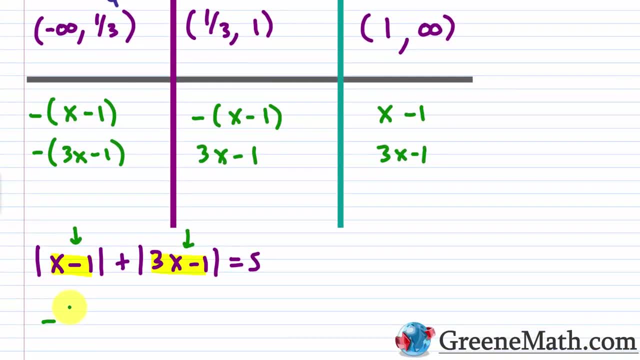 So this guy right here is going to be replaced with its negative. So the negative of x, x minus 1, then plus, this guy is positive. so we just say 3x minus 1, and this equals 5, okay. 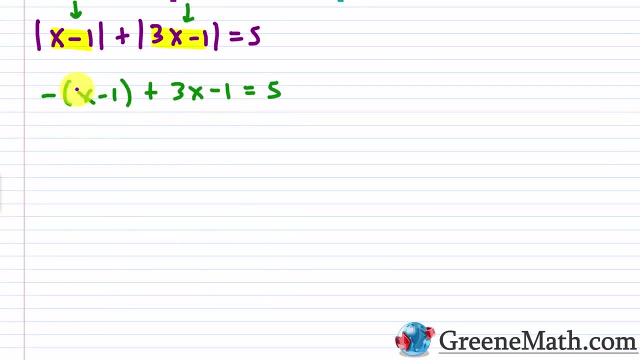 So let's go ahead and solve this and then we will come back up. So distribute the negative to each part. You have negative x, and then plus 1, then plus 3x and then minus 1 equals 5.. So we know that 1 minus 1, those would cancel, right. 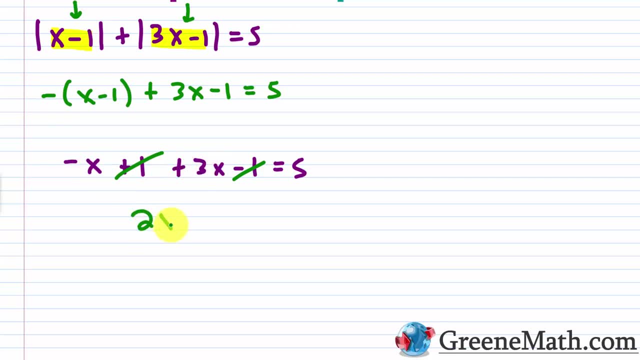 That's basically 0.. So you'd have negative x plus 3x, which is 2x, and this is equal to 5, okay, So what I'm going to do from here is I'm going to divide both sides of the equation by 2.. 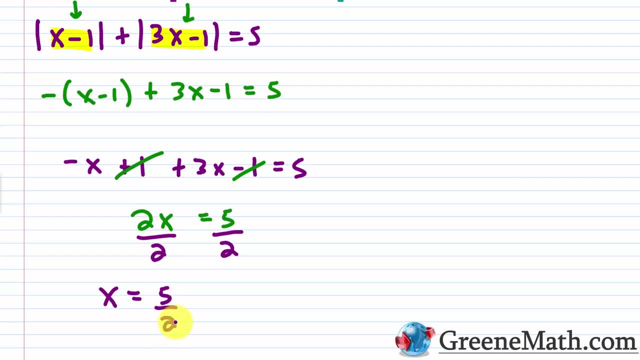 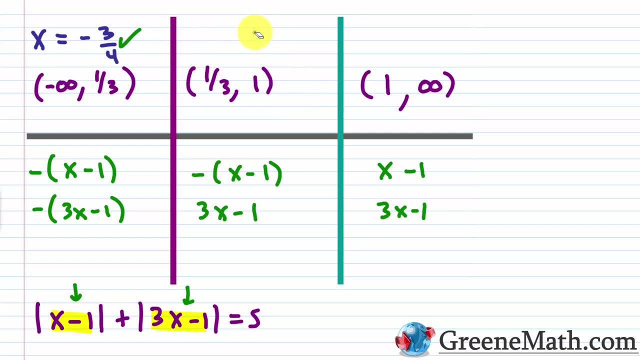 And I'm going to get that x is equal to 5 halves. Now let me erase everything. Let me paste this in, So we have x equals 5 halves. Let me kind of do this in a different color so it doesn't get confusing. 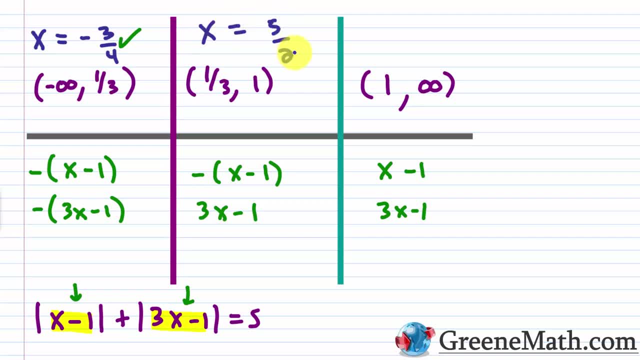 So x equals 5 halves. Does 5 halves lie in the interval which is between 1 third and 1, right, with neither included? No, it doesn't, because 5 halves is 2.5.. So this is the solution we're going to reject, right? 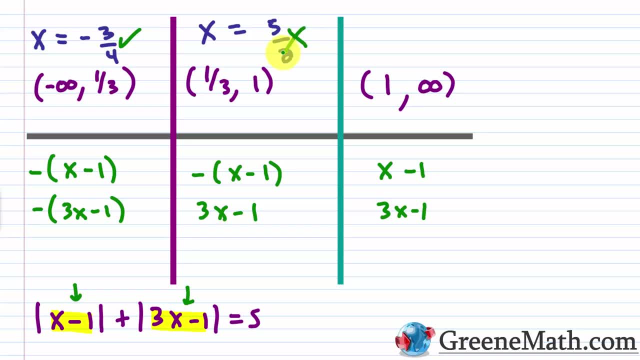 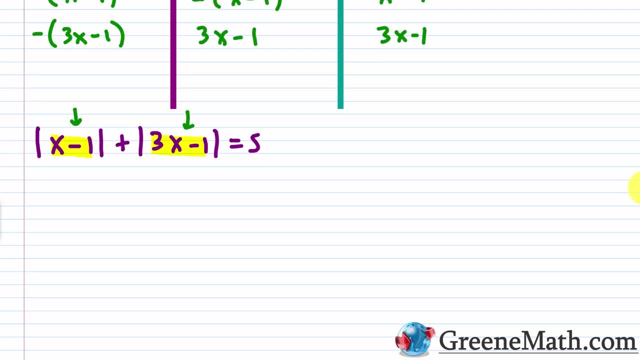 We're going to reject this solution. Now. we're going to move on to this interval right here, which is anything larger than 1.. So in this interval, both of these are positive. So what I'm going to do is I'm going to drop the absolute value bars in each case and just 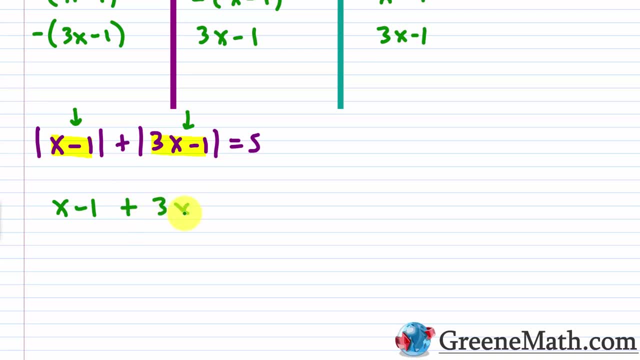 write what I have. So I'd have x minus 1 plus 3x minus 1, and this is equal to 5.. So then I would add x plus 3x, that's 4x Negative. 1 minus 1 is negative 2.. 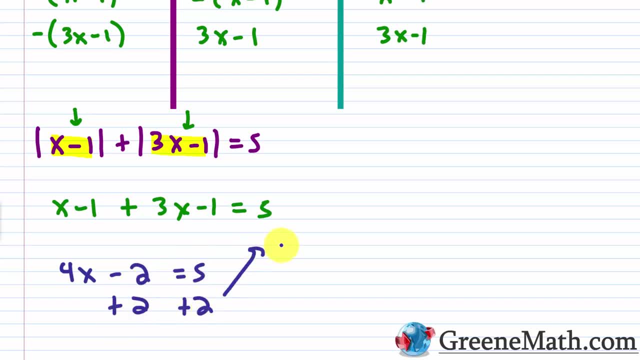 This equals 5.. We would add 2 to both sides of the equation, And so we would have that 4x is equal to 7.. We can divide both sides of the equation by 4 and find that x is equal to 7 fourths okay. 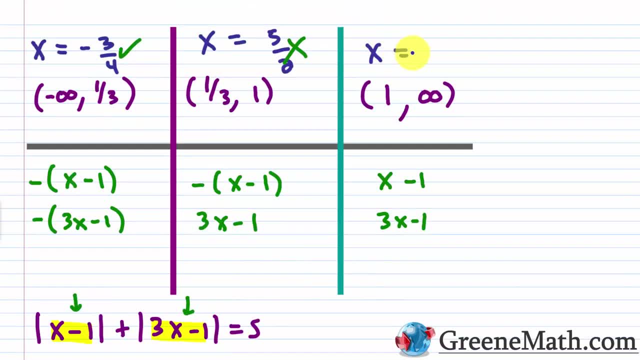 So let me erase this once again and we'll say: x equals 7 fourths. okay, So is 7 fourths in the interval again anything larger than 1?? Well, yes, it is. 7 divided by 4 in decimal form is 1.75, so that's clearly larger than 1.. 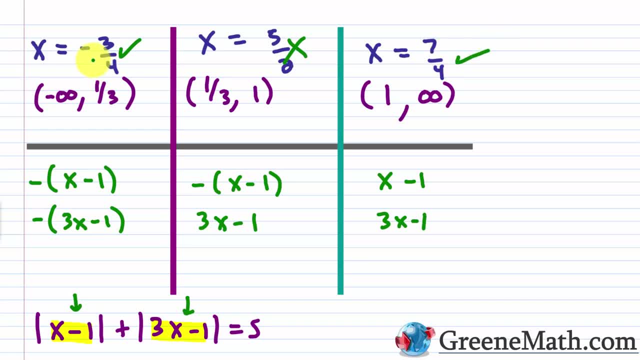 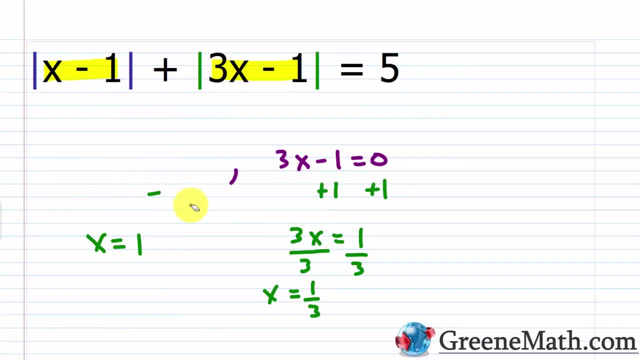 So your two solutions here. let me just kind of check this off. You would have that x is equal to negative 3 fourths or x is equal to 7 fourths. So let's go back up here- I'm just going to erase this- and we'll say that x is equal to negative 3 fourths and 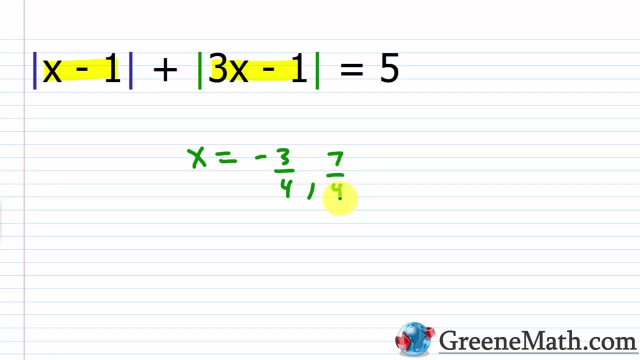 then also 7 fourths right, And we rejected 5 halves. That didn't work. You can check this if you want. You can even check 5 halves and prove that to yourself, that it doesn't work If you plug in negative 3 fourths here, so you have the absolute value of negative 3. 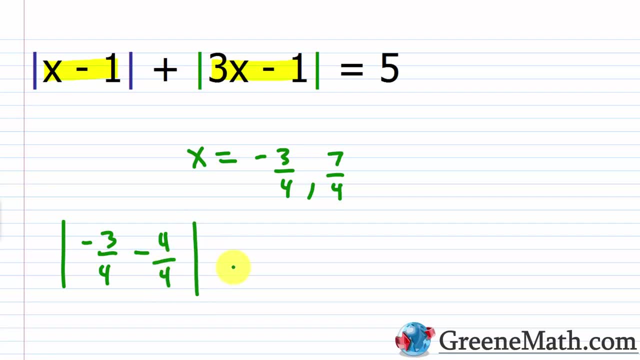 fourths minus 1,. so minus 4 fourths. I'm just getting a common denominator Then plus the absolute value of 3 times negative 3 fourths. okay, then minus 1, and then this is equal to 5.. 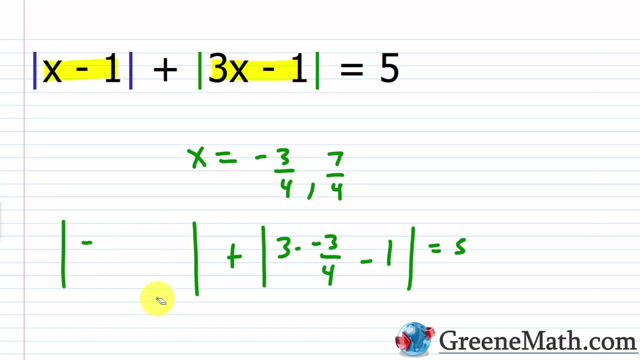 Negative 3 minus 4 is negative 7, so this would be negative 7 fourths. And then if I took the absolute value of that, I'd have 7 fourths okay. So this would be 7 fourths, so that works okay. 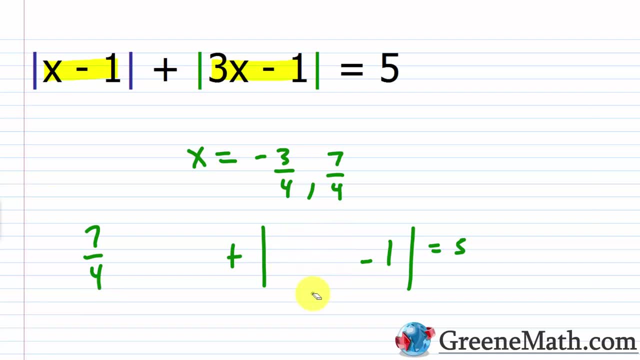 And then this guy right here: 3 times negative. 3 is negative 9, so this is negative 9 fourths, Again, getting a common denominator. just write this as 4 over 4.. Okay, Negative 9 minus 4 is negative 13,. so you'd have negative 13 fourths. okay, so you'd have. 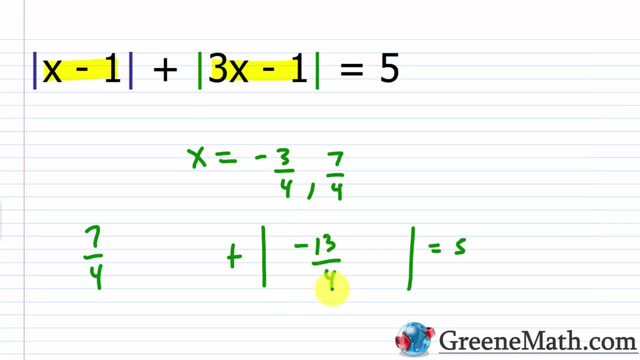 negative 13 fourths. Take the absolute value of that, you get 13 fourths. okay, So this is 13 fourths here, And what do you get? 7 plus 13 is 20 over the common denominator of 4,. you would get 5, right. 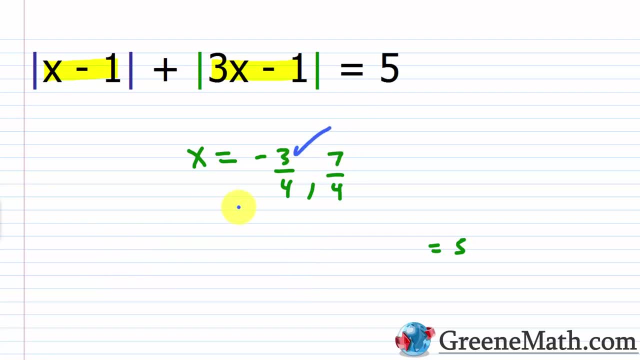 So you know, this one would work itself out. So this one checks out. All right, so let's check the other one. So the absolute value of you'd have 7 fourths minus for one. I'm going to put 4 fourths. 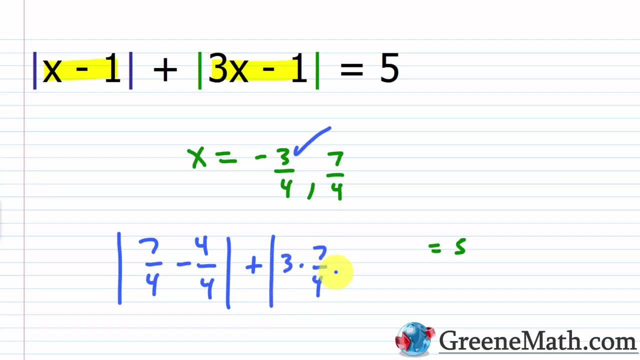 and then plus The absolute value of 3 times 7 fourths. minus again for one, I'm going to put 4 fourths. So what do we have here? 7 minus 4 is 3, so over the common denominator of 4, this would be 3 fourths. 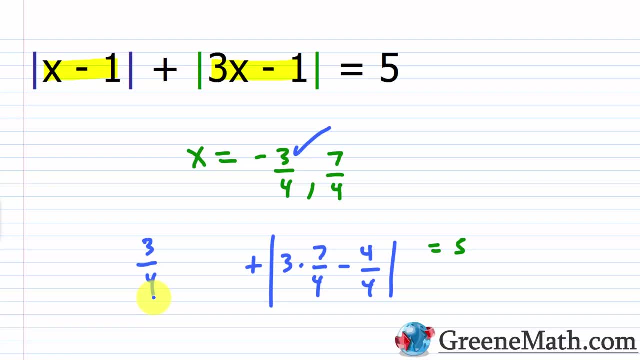 Absolute value of 3 fourths is 3 fourths, okay. So that's 3 fourths. Then this guy here, 3 times 7 is 21,. so you would have 21 here. Then 21 minus 4 is 17,. so you would have 17 fourths, okay. 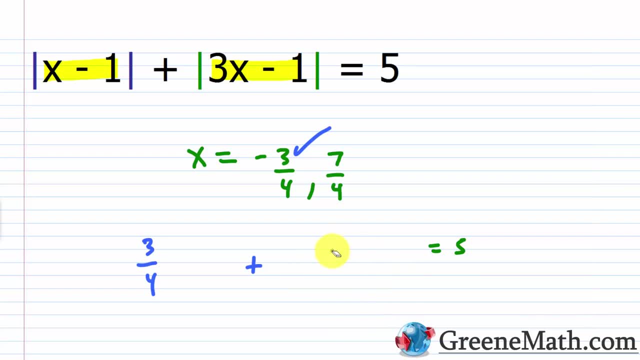 17 fourths. Absolute value of 17 fourths is 17 fourths, And you see that this works right. 3 plus 17 is 20.. 20 over 4 is 5, so you get 5 equals 5, so this works out as well. 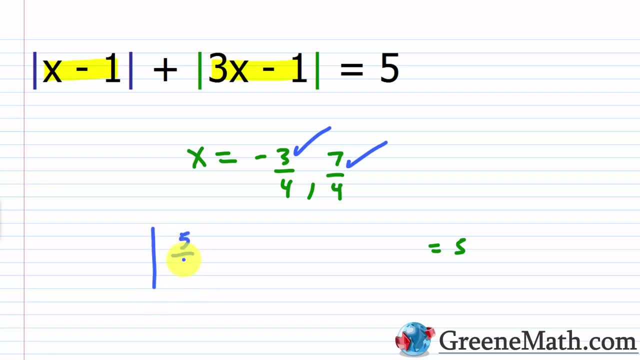 So you can also do 5 halves and prove that it doesn't work. So you'd have 5 halves minus. in this case I'm going to write 1 as 2 over 2. And then plus, you'd have 3 times 5 halves and then minus 1.. 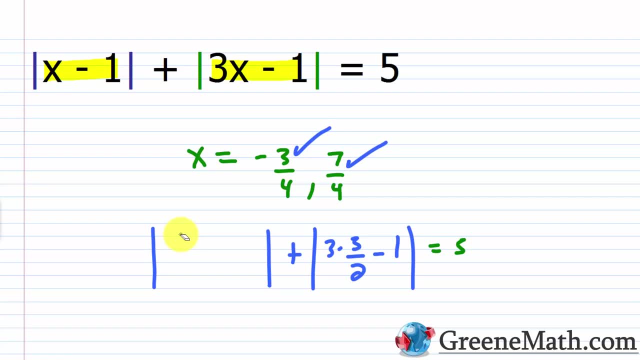 So we know that this would be what. This would be: 3 halves, This would be 3 halves. Absolute value of 3 halves is 3 halves. So this would be 3 halves. And then this guy, 3 times 5 is 15, so you'd have 15 halves. 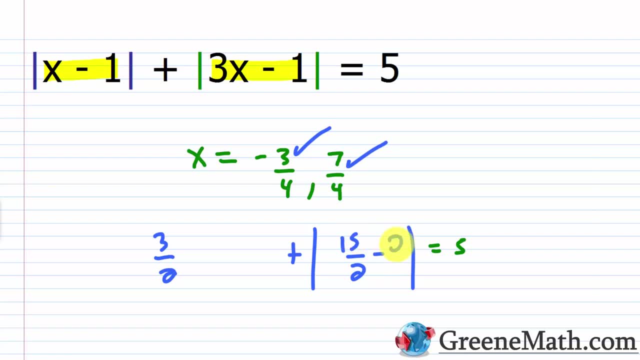 Again, I'm going to write this as 2 over 2.. 15 minus 2 is 13,, so you'd have 13 halves. Absolute value of 13 halves is 13 halves. So in this case you'd get 3 plus 13,, which is 16.. 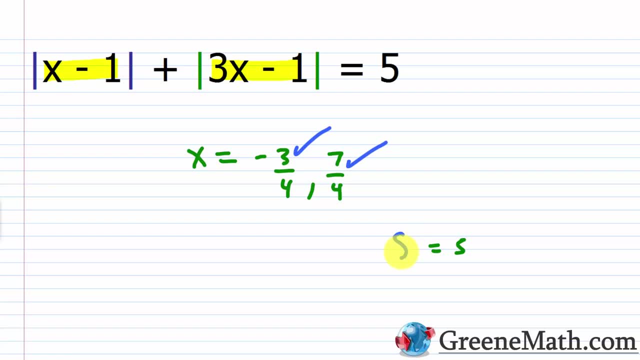 And so you'd have 16 over 2, which is 8.. So you get 8 equals 5,, which is false. okay, That's false. So that solution where x equals 5 halves again. you've got to reject this. 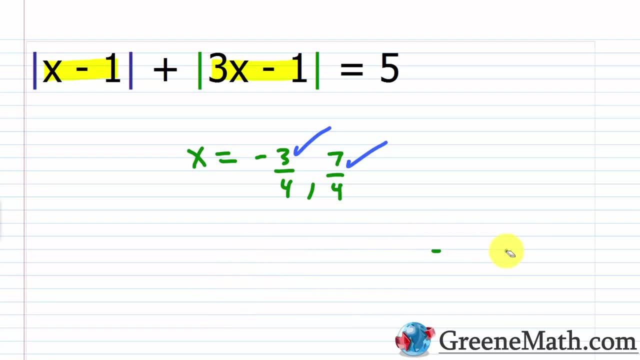 This does not work okay, And we found that because it wasn't in the interval. we knew it wasn't going to work. Now let's talk a little bit about the alternative method to solve this. This is one that I don't recommend, because it just takes a lot more time. 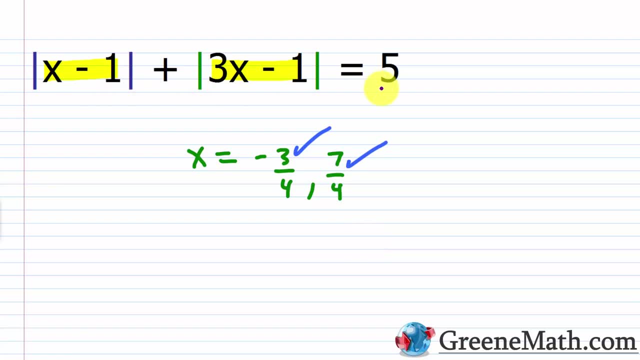 So what you can do is you can consider all the cases that you would be presented with this. So, in other words, you can consider if this expression is positive and this expression is positive, you would just have x minus 1 plus 3x minus 1 equals 5, okay. 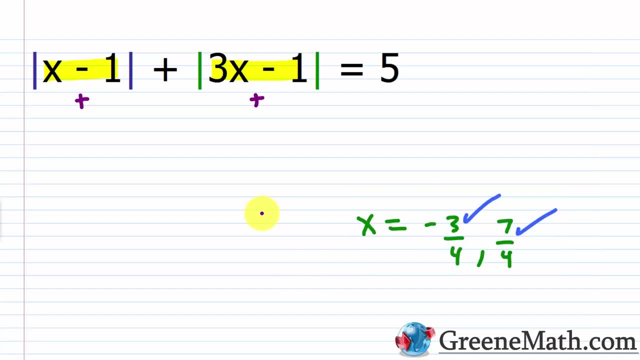 So that's one scenario that you would encounter. Okay, Then another scenario would be this one's negative and this one's positive. So in other words, I would put a negative out in front of this and say the negative of x minus, 1 plus, and then this guy's positive, so 3x minus 1, and this equals 5.. 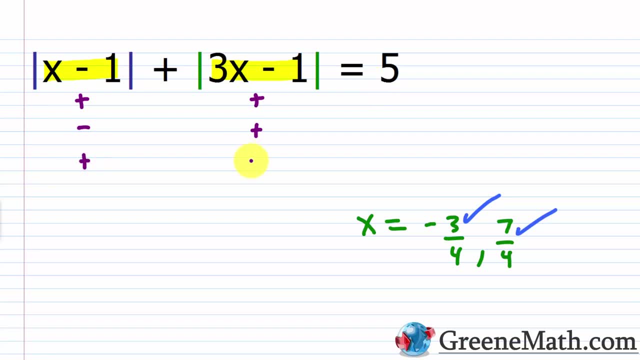 So I'd solve that equation Right, And you keep going. So this would be positive and this would be negative, and this would be negative and this would be negative. So you basically have four equations to set up and solve, but then you get extraneous. 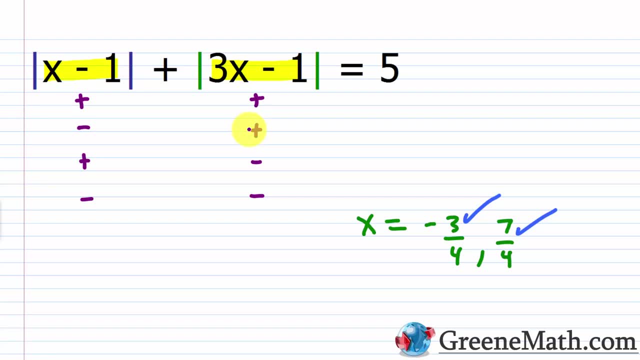 solutions. So you have to go back and check each one of those. okay, And with our method, we really don't need to check. We just need to verify that our solution lies in the interval that we've created and that we're basically good to go. okay. 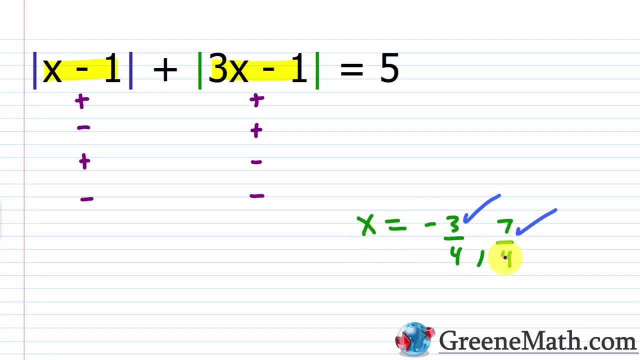 So, once more, the solution here is that x equals negative 3 fourths or 7 fourths. All right, let's go ahead and take a look at another one of these. So we have the absolute value of 5x plus 3, then minus the absolute value of 2x minus. 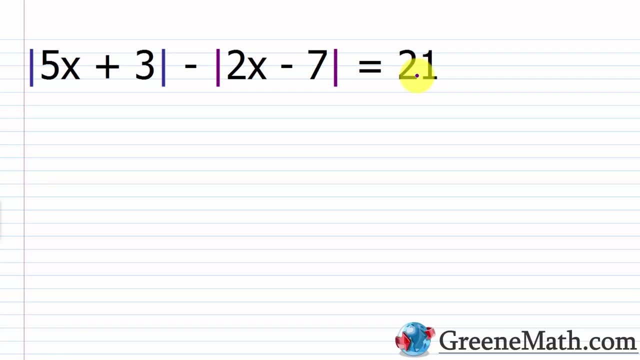 7, and this equals 21.. So again, it's the same thought process. I'm thinking about where this guy is 0 and where this guy is 0. I'm using that to kind of set up intervals on my number line. 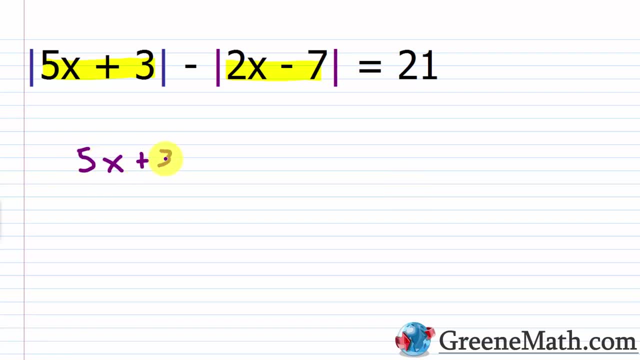 So we'd have 5x plus 3, and we'd say: where is that equal to 0?? So I would subtract 3 away from each side of the equation. I would get 5x is equal to negative 3, divide both sides by 5, and I get that x is equal. 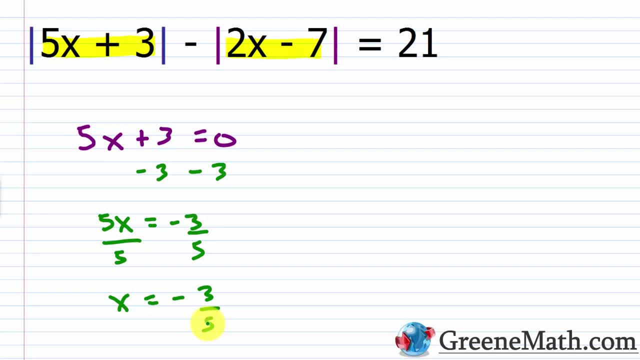 to negative 3 fifths. okay, So that's going to be one of those guys. Then for this guy right here, where is 2x minus 7 equal to 0?? Let's add 7 to both sides of the equation. 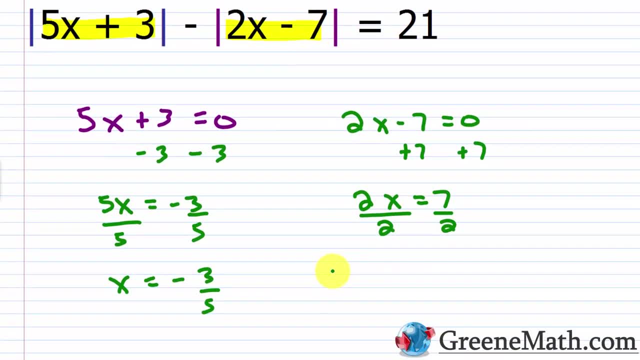 We get 2x is equal to 7.. Divide both sides by 2.. We get x is equal to 7 halves okay. So basically I'm going to have an interval that is anything less than negative 3 fifths. 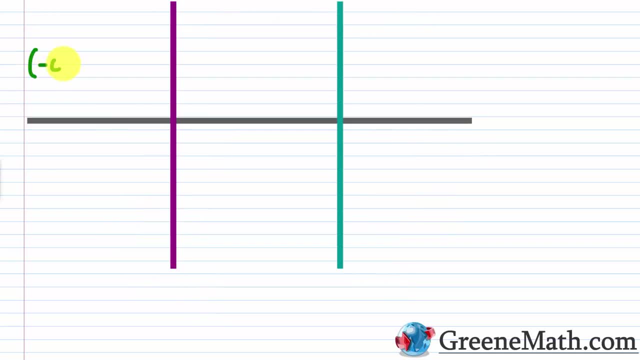 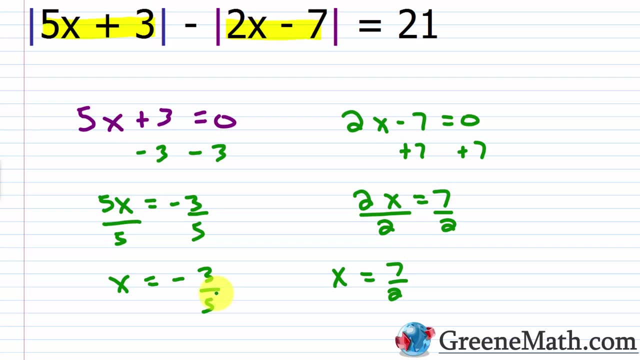 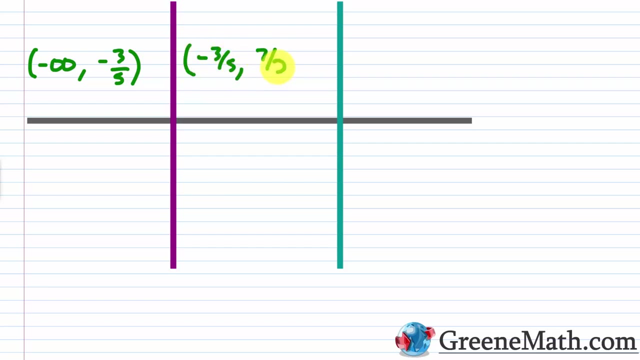 So let's write that first. So we'll put negative infinity here up to, but not including, negative 3 fifths. Then I'm going to have an interval between negative 3 fifths and 7 halves, with neither included. So you have negative 3 fifths and 7 halves. again neither one's included. 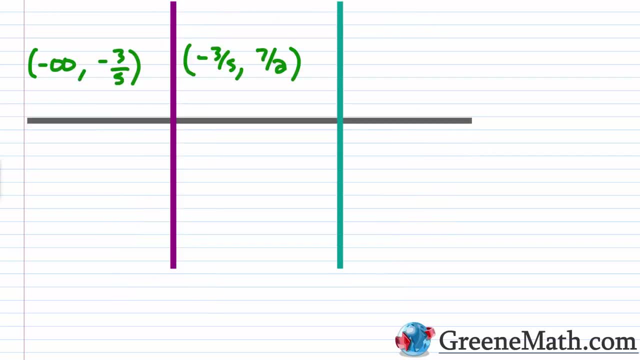 And then, lastly, we have an interval where we're greater than 7 halves. okay, So, where we're greater than 7 halves, Okay. so let's rewrite our absolute value equation, So we have the absolute value of 5x plus 3, and then minus the absolute value of 2x minus. 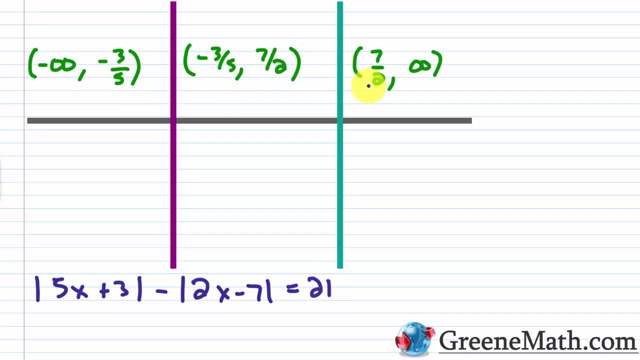 7. This guy is equal to 21. So again, I'm just going to look into each interval and decide where each expression is positive and negative. Again, if it's positive, I can just kind of drop the absolute value bars. 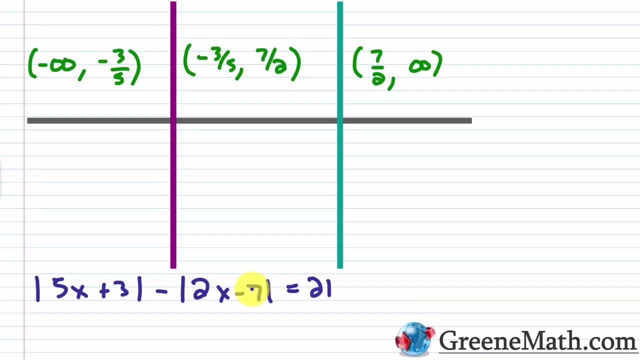 If it's negative, I can drop the absolute value bars, Wrap it in parentheses, Wrap it in parentheses and put a negative out in front right to change it into its opposite. So we know that if we're less than negative 3 fifths, both of these expressions are going. 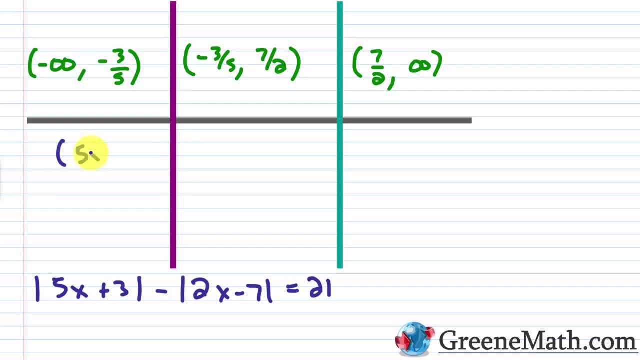 to be negative, right? So 5x plus 3, I'd wrap that in parentheses. put a negative out in front. 2x minus 7, I'm going to wrap that in parentheses. put a negative out in front. 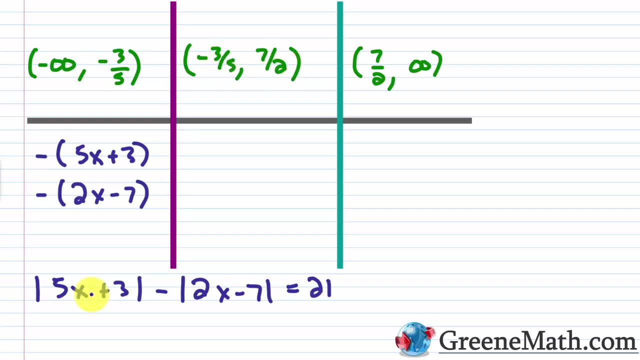 If I'm between negative 3 fifths and 7 halves, I know this guy right here is going to be 0 at negative 3 fifths. Okay, Okay. So negative 3 fifths- That guy's positive right. 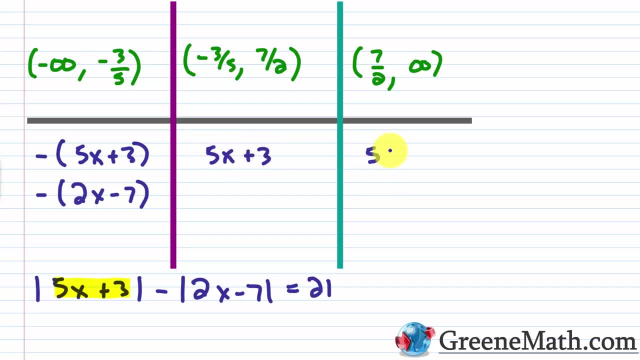 So 5x plus 3 is positive, And I can go ahead and just say it's going to be positive in this interval as well. right Now, this guy, right here, this 2x minus 7, this guy is going to be 0 when x is 7 halves. 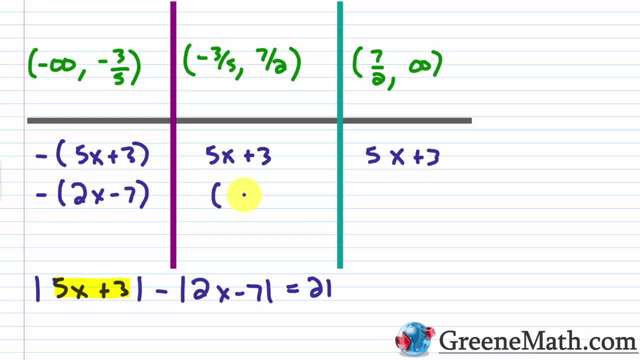 So it's still going to be negative in this interval here. So we would wrap this in parentheses and put a negative out in front. And again, in this interval it's positive, because everything's positive once we get larger than 7 halves. 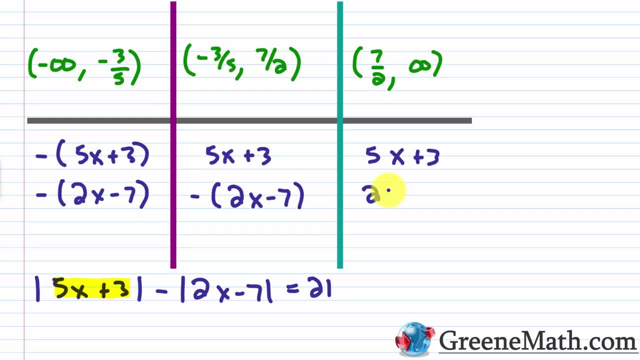 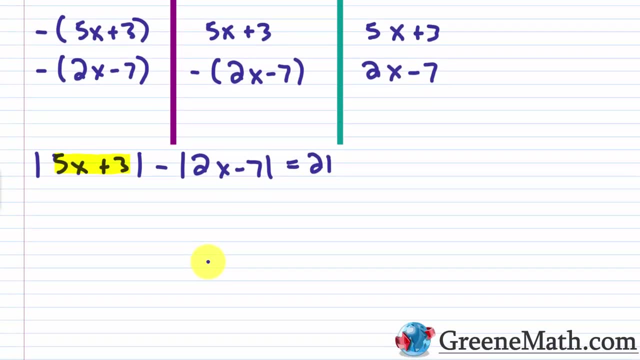 Okay, this guy 0. So we'll say this is just 2x minus 7.. Okay, So let's go through the possibilities, Let's scroll down, Let's think about the first one. So, all the way to the left, I'm going to. 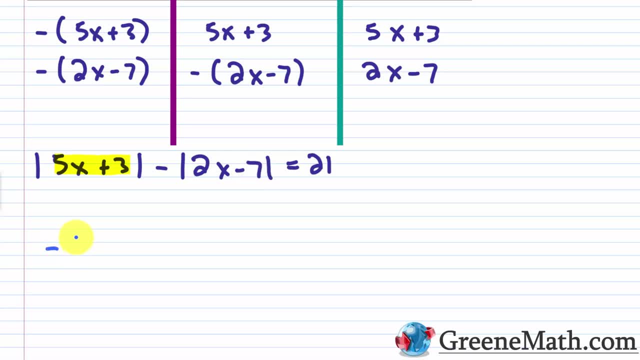 replace each one of these with their opposite. So I'm going to have the negative of 5x plus 3. And then minus. you've got to be very careful, because this is a minus here, And then you're putting a negative out in front. So minus a negative is really plus a positive, right? 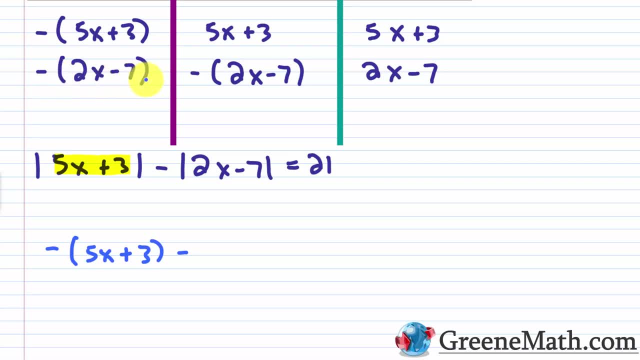 So minus a negative, and then times the quantity 2x minus 7, I'm going to put plus, Okay, So plus 2x minus 7.. Okay, And then this equals 21.. All right, So I'm going to distribute this negative. 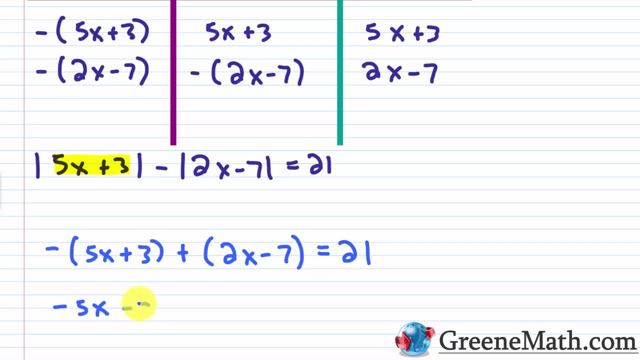 to each term. I'll have minus 5x and then minus 3, and then plus 2x and then minus 7.. This equals 21.. Okay, Let me scroll down and get some room going. We'll come back up. So this guy right here. 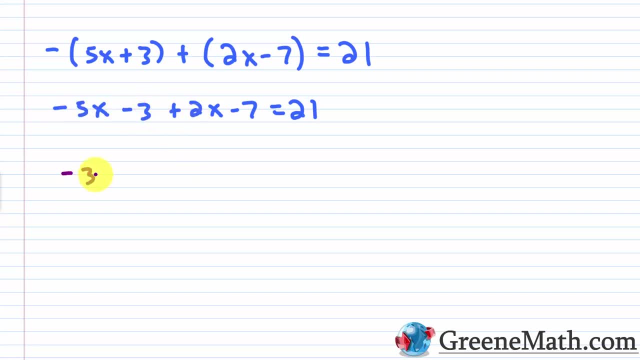 so negative 5x plus 2x, That's going to be negative 3x. And then negative 3 minus 7 is negative 10.. This equals 21.. Let's add 10 to both sides of the equation: We're going to get negative. 3x is equal to 31.. We're going to 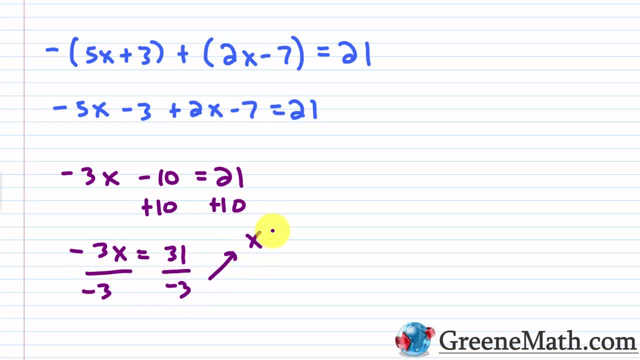 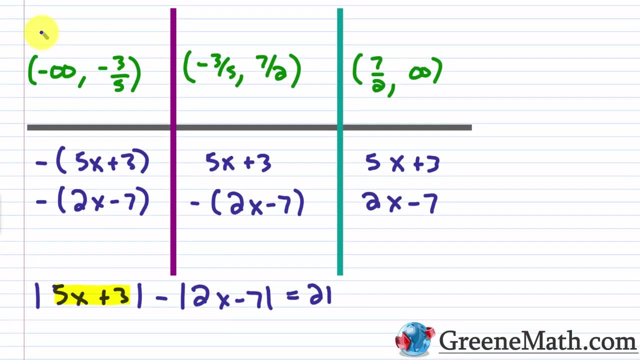 divide both sides of the equation by negative 3. And we're going to get that x is equal to negative 31 thirds. Okay, So let's copy this. So let me just write that in here: X equals negative 31 thirds. Okay, Negative 31 thirds. So is this valid? 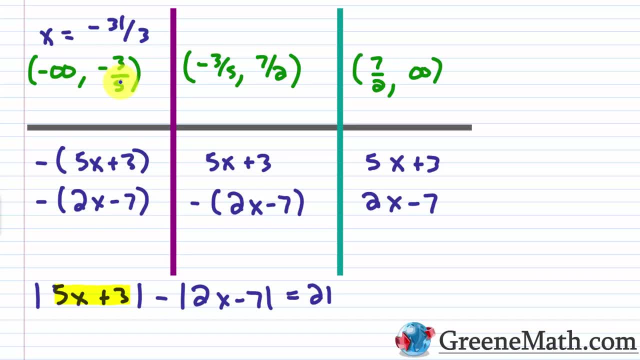 You just need to ask yourself the question: does it lie in this interval? And the answer to that is yes, right, Negative 31 thirds is more negative, or to the left of negative three fifths. So you can clearly see it would be in this interval. So, this guy, we'll go ahead and check it off and say: 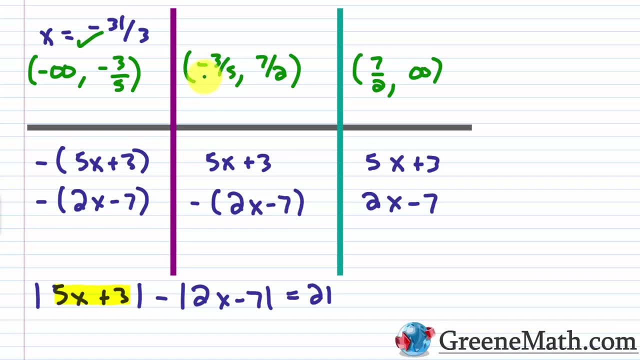 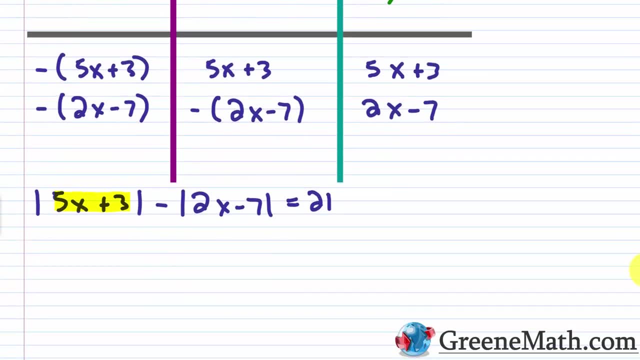 that's a valid solution. All right, Let's talk about, in this interval here between negative three fifths and seven halves. So this guy's positive and this guy's negative. So let's scroll down a little bit and we'll say that we have 5x plus three. Again, if I have a minus a, 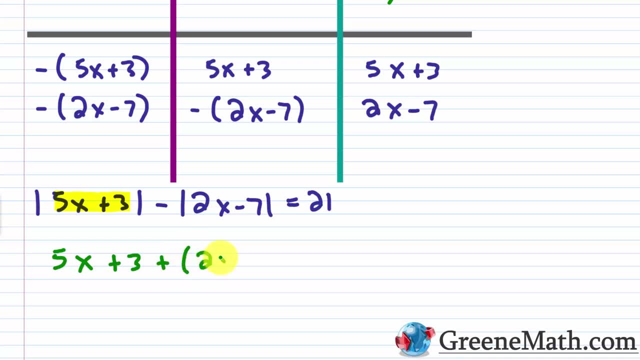 it's plus a positive. So you just say plus. there again two X minus seven, And I really don't need the parentheses, I can just drop them And then this equals 21.. So let's just solve this real quick. I'm just going to scroll down and get a little room going. We'll come back up. So 5x plus. 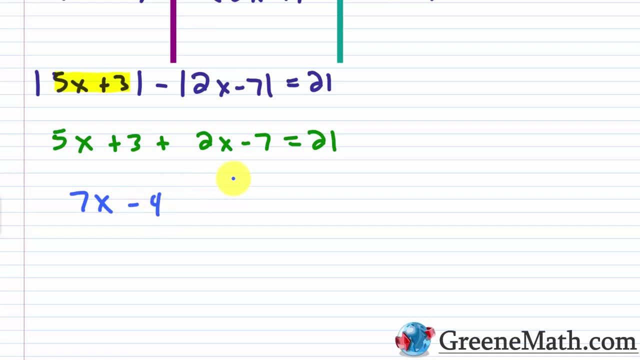 two X is seven X. three minus seven is negative four. This equals 21.. And let's go ahead and add four to both sides of the equation, So we have seven X is equal to 25.. Let's divide both sides: is equal to 25 sevenths. All right, So let me kind of copy this real quick And I'm just going. 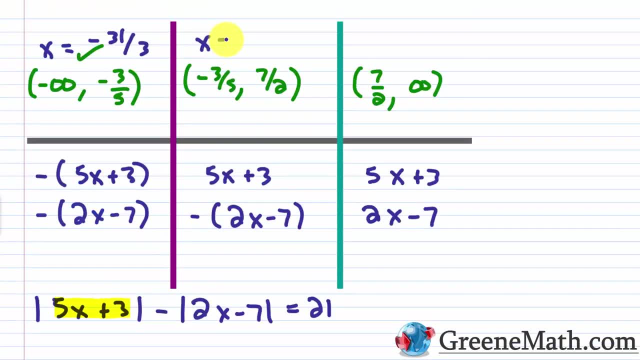 to erase all this work, We're going to go back up. So again, X is equal to 25 sevenths, So 25 sevenths. So is that in the interval again between negative three fifths and seven halves, Well, negative three fifths is basically negative 0.6 as a decimal. Seven halves is 3.5.. Okay, 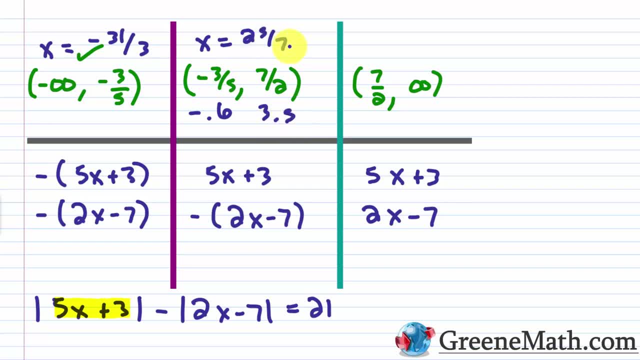 And if I think about 25 sevenths, that's a little bit larger than 3.5.. It's 3.571.. If you wanted to kind of go to three decimal places, So it is larger than 3.5.. So it's outside of this interval. So we're going to end up. 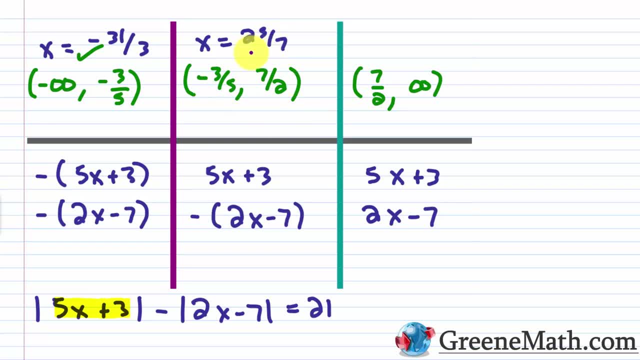 rejecting this solution. Okay, It's not going to work, So let me do that in red. I'm going to reject this, And so now we just have to check this interval here. So everything's positive, So I can just drop the absolute value bars, So we kind of go down and do that, So we would have five X plus. 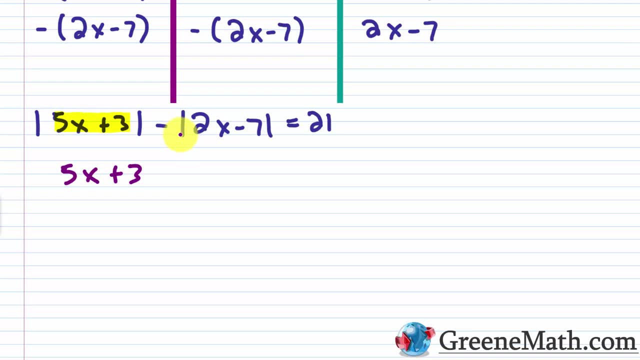 three, And then basically, you're subtracting away this whole thing. Okay, You've got to be careful there. So what I'm going to do is I'm going to say minus- I'm going to wrap this in parentheses- two X minus seven, because again, this whole thing's being subtracted away. Don't make the. 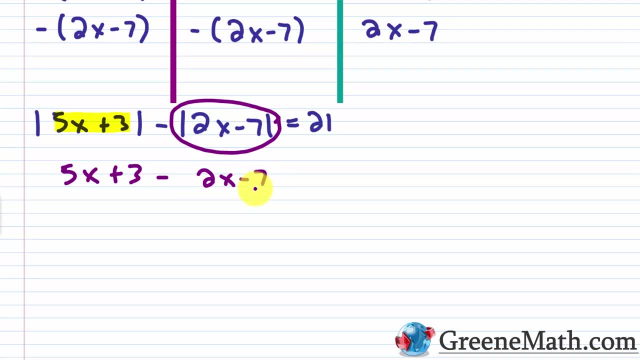 mistake of just putting a minus two X and then leaving this as negative seven, because this has to be changed And so does this. Okay, You got to be very careful there. So then this equals 21.. Okay, So I'm going to go ahead and say: five X minus two X is three X. 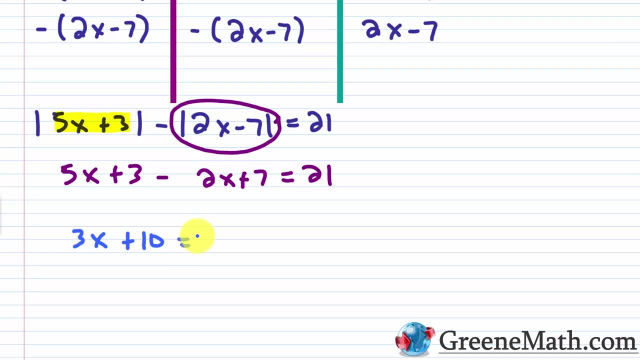 And then three plus Seven is 10.. So plus 10 is equal to 21.. Let's go ahead and subtract 10 away from each side of the equation And we'll say that three X is equal to 21 minus 10 is 11.. Divide both sides by three. 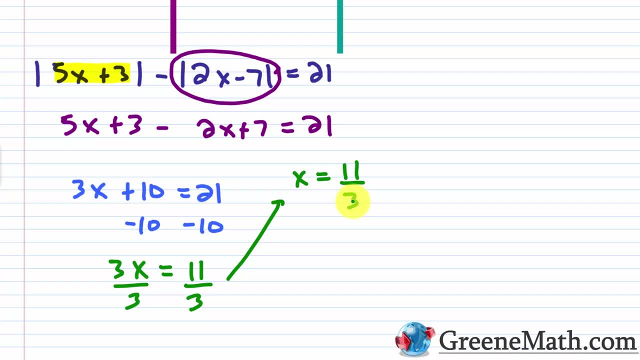 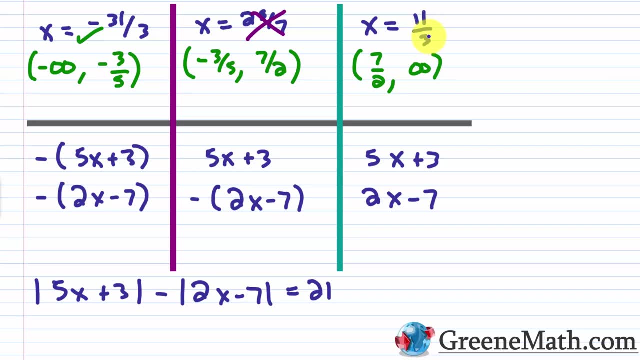 We're going to get that X is equal to 11 thirds. Okay. So once again, let me erase everything. All right, So we found that X is equal to, again, 11 thirds. Okay, So is 11 thirds in this interval. 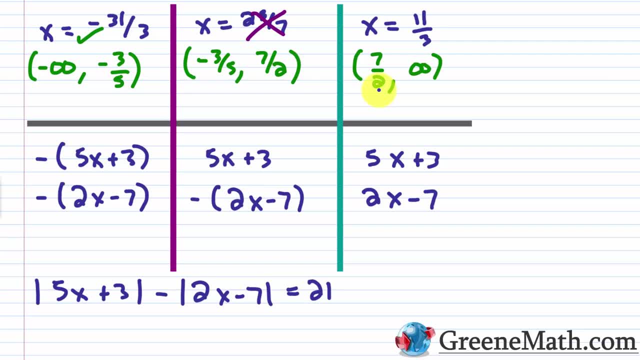 Well, seven halves is 3.5. So it needs to be larger than that. So if you bunch up 11 divided by three in a calculator, you get 3.6, where the six repeats forever. Okay, So that is going to be larger than 3.5.. So this guy is going to work out as a 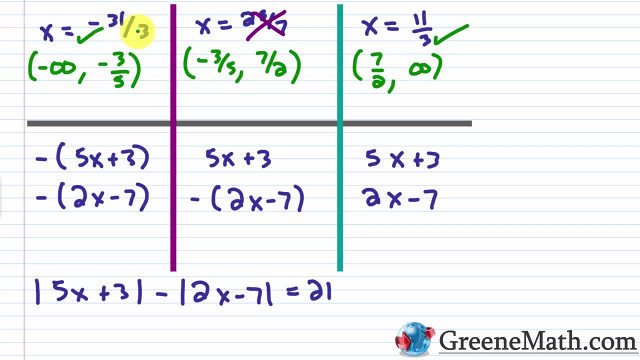 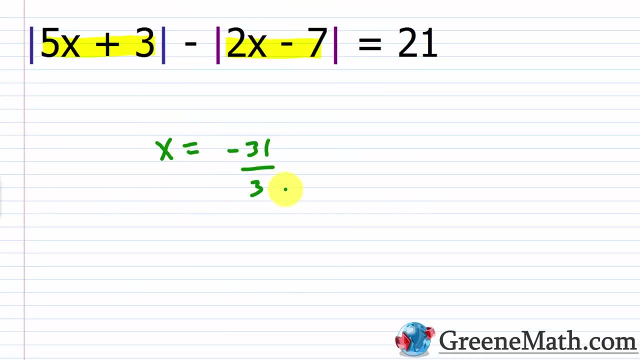 solution. So the two solutions are going to be: X equals negative 31 thirds and then X equals 11 thirds. So let me go back up So we'll say that X is again equal to. we have negative 31 thirds and also 11 thirds. All right, So let's wrap up our lesson and look at another common type of 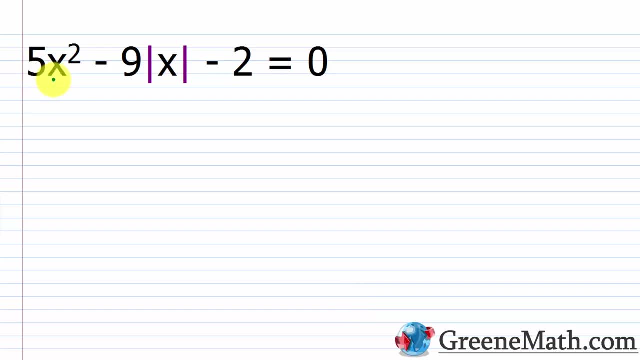 problem that you'll see. So let's say we ran out of time, We ran out of time. We ran out of time. We ran into something like this: We have five X squared minus nine times the absolute value of X minus two, and this is equal to zero. So in this particular case, we have this absolute value. 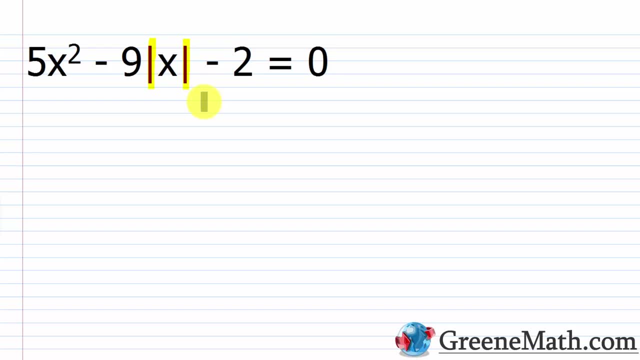 operation that's kind of in the middle of our equation and we can't really isolate it. So there's kind of two different ways to solve this. One of them is just to consider the two cases and then just kind of go back and think about if the solutions that we get work right. So you just 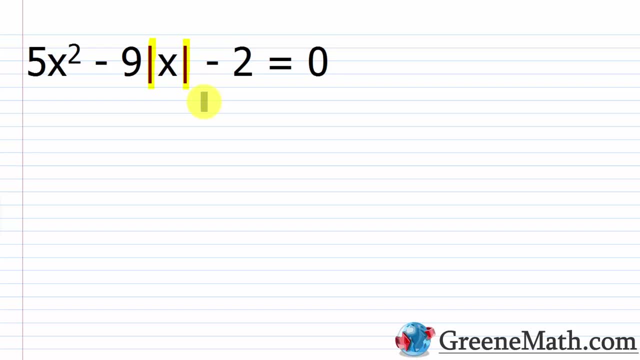 plug them back in. The other one would be to kind of make sure that we have the solution that we need to solve, So you can make a little substitution and then you can consider if things are valid or not from that. So let's try it the first way, And then I'll show you the substitution. 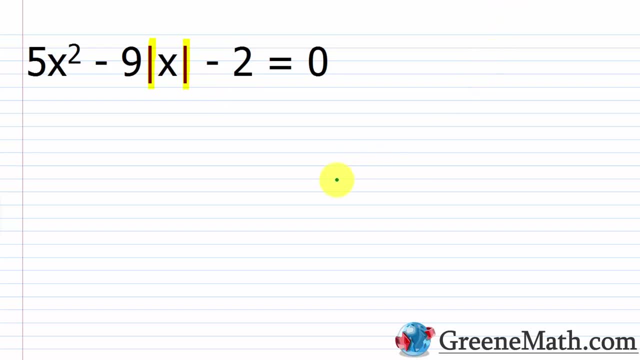 method. I prefer the substitution method on this, but you can do it either way. So there's two cases here. One case would be that this value here is going to be positive. So in that case we just remove the absolute value bars, So you would have five X squared minus nine X minus two equals zero. 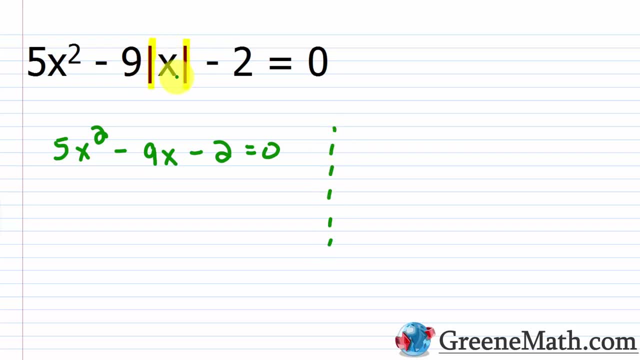 And then the other case- kind of the case over here- would be: let's say this expression was negative. So then I'd remove the absolute value bars and I would make X negative, X right. So we would have five X squared minus nine. It's being multiplied by this. 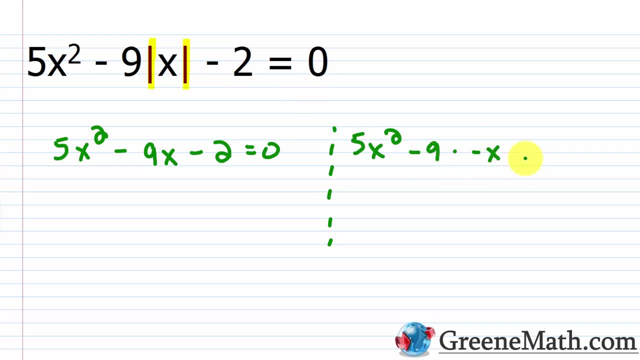 and I'm multiplying it by the negative of X, and then minus two, and this equals zero. Of course we could simplify this, because negative times negative is positive. So I can now write this as: plus nine X. Okay, So plus nine X. Let me kind of tighten this down a little bit. 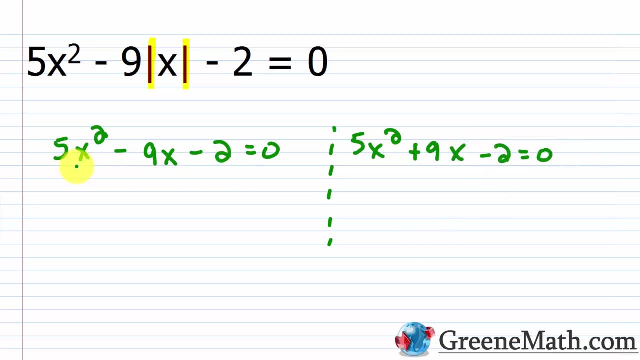 Just move that over there, Okay. So let's start over here on the left. So this is something we can factor over here on the left. So let me kind of set this up and we'll factor this guy real quick. So I know that this is going to be five- X and this is going to be X because this is a prime number. 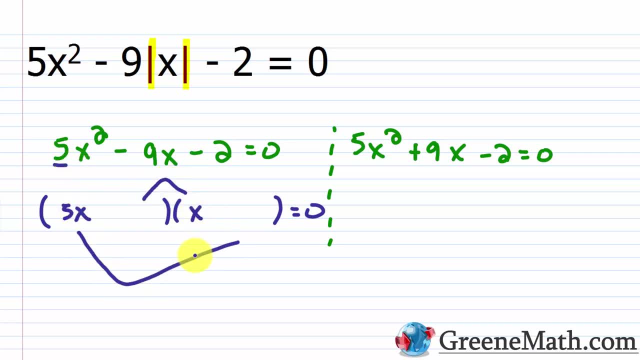 here. So I need to make sure the outer and the inner work itself out. So I'm looking for what. I'm looking for? a middle term of negative nine X and I'm looking for a final term of negative two. So when we think about negative two, we know something's got to be positive and something's. 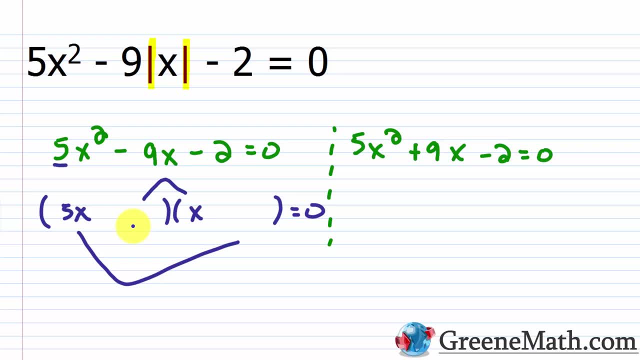 got to be negative. Okay, So we also know that the factors there could be, you know, one and negative two, or it could be negative one and positive two. Okay, So let's say I put my negative two here and my positive one here. Would that work? So in this case, five X times negative two would give. 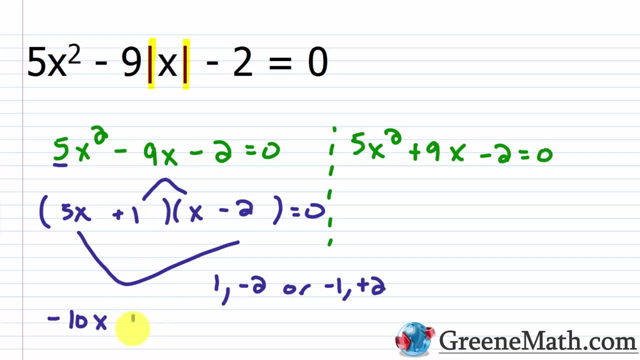 me negative 10 X and then one times X would be plus X. So this does work itself out: Negative 10 X plus X would be negative. And then if you think about one times negative two, of course that's negative two. So this is. 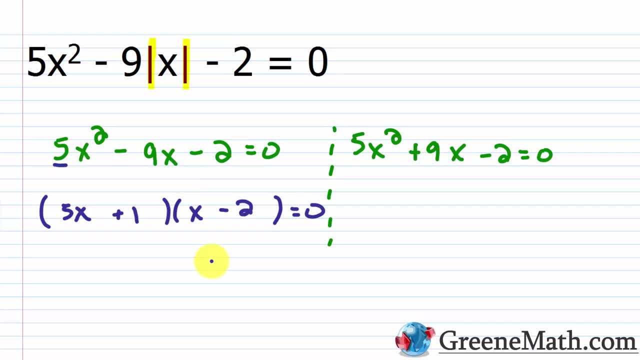 our correct factorization. here And now we can just solve this pretty easily. We're going to take each factor and set it equal to zero. So five X plus one equals zero, And then we're also going to have that X minus two is equal to zero. Let me kind of scroll down real quick. get a little room. 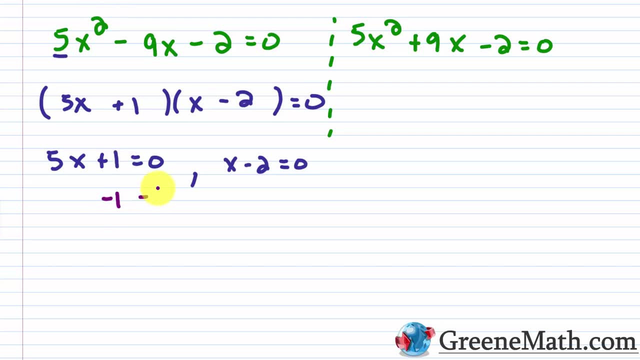 going, And so, to solve this one, I'm going to subtract one away from each side of the equation. I'll have five. X is equal to negative one. divide both sides by five and I get X is equal to negative one. fifth: Okay, Then over here, let me add two to both sides of. 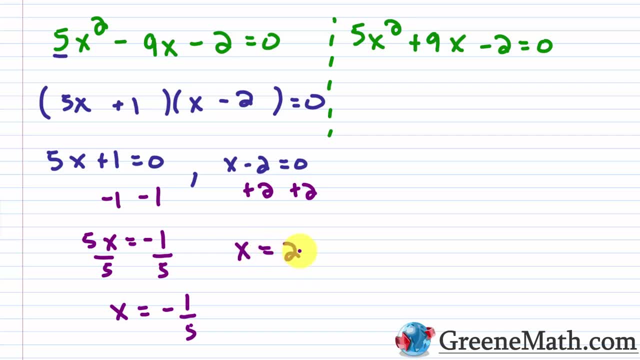 the equation And I get that X is equal to two. Okay, Now, these are just proposed solutions. We actually need to check them in this scenario. So let me erase all this and I'm just going to copy these. So I'm just going to put this over here. We have: X is equal to two and then common negative. 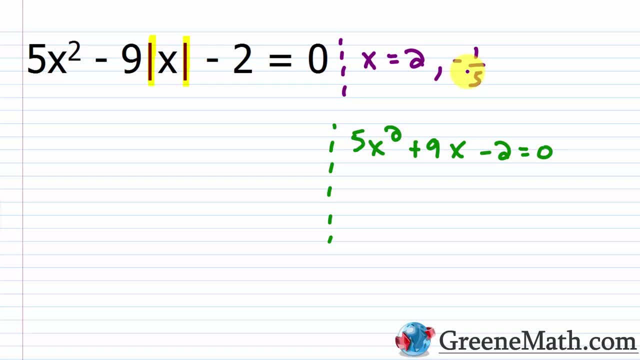 one, fifth. We'll check them in a minute. We're going to find that some of these won't work, So let's move this over here and let's work on this Now. we'll get the solutions for and then we'll check everything at once. Okay, So for this guy, we can also solve this with. 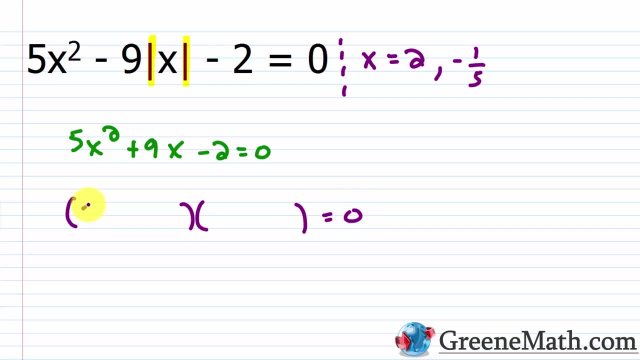 factoring. So let's go ahead and set this up So we can again do five, X and X Again. I'm looking for the outer and the inner, such that I get a positive nine X as my middle term and a negative two as my final term. So instead of doing a negative two here, I'm going to do a 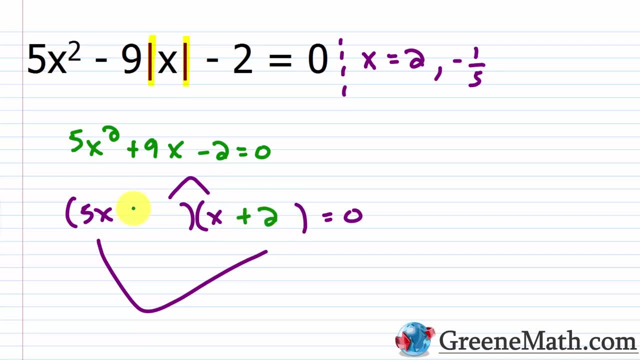 positive two, And instead of doing a positive one, I'm going to do a negative one, right? Because my outer would be 10 X And my inner would be minus X. So 10 X minus X would give me my positive nine X and then negative. 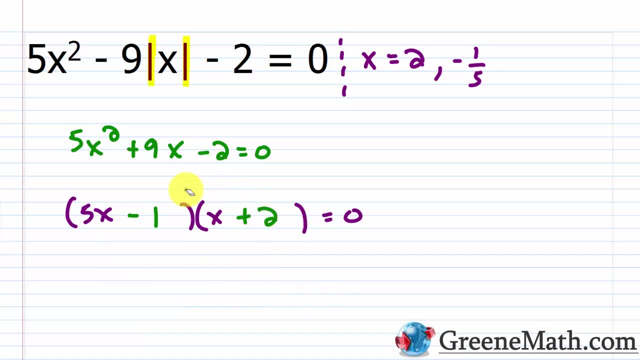 one times two would be negative two. Okay, So we're good to go there, All right. So now I'm just going to set each of these equal to zero. So five X minus one. if that equals zero, we're going to find that we add one to each side of the equation, We'll get that five X is equal. 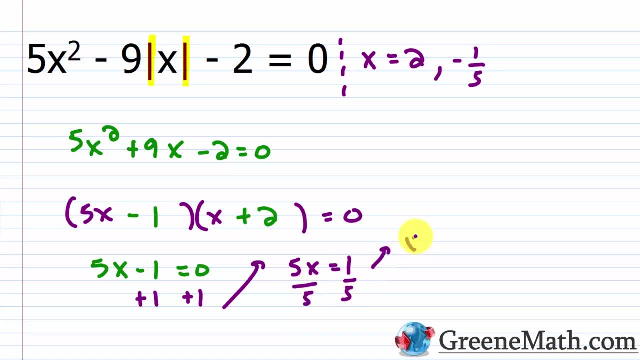 to one. divide both sides by five and we're going to get that X is equal to one fifth. Okay, So let me just write that in here. So we have one fifth, And I'll just erase this. We don't need this information anymore. And then we also have X. 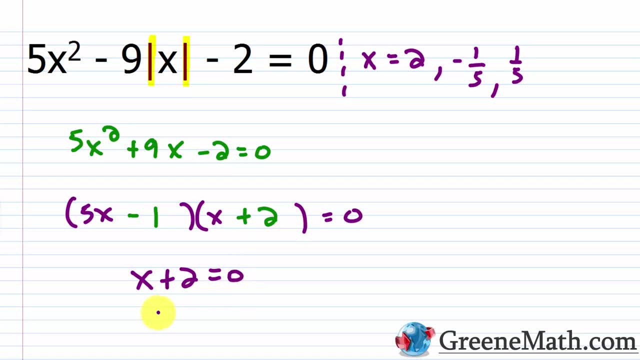 plus two, We're going to set that equal to zero. Of course, that gives me a solution. If I subtract two away from each side, that X is equal to negative two. Okay, Let's put negative two in there, All right? So let's erase everything. And now we just want to check our solutions. 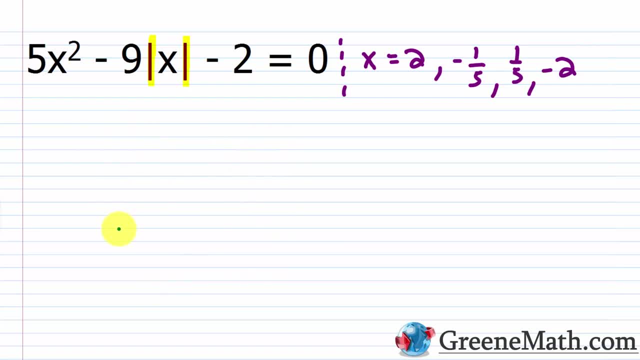 and see what works and what doesn't. Okay, So we have five times for X, I'm going to start by plugging in a two, So you'd have two, that guy squared, then minus nine times the absolute value of one Right Plug in. and then for X, then minus two, and this equals zero. Okay, So two squared is. 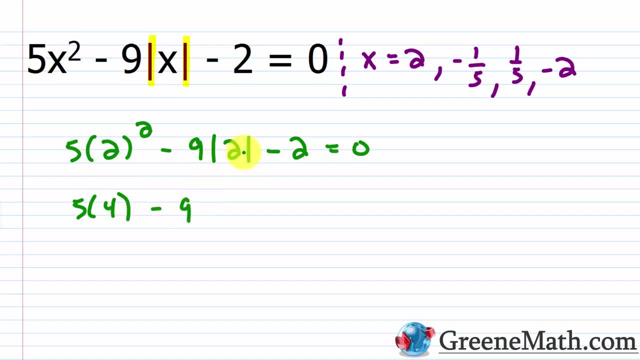 four, So you'd have five times four, then minus nine times the absolute value of two. The absolute value of two is two, So nine times two, then minus two, and this equals zero times four is 20.. Then minus nine times two is 18.. Then minus two, and that should equal zero. And this is going. 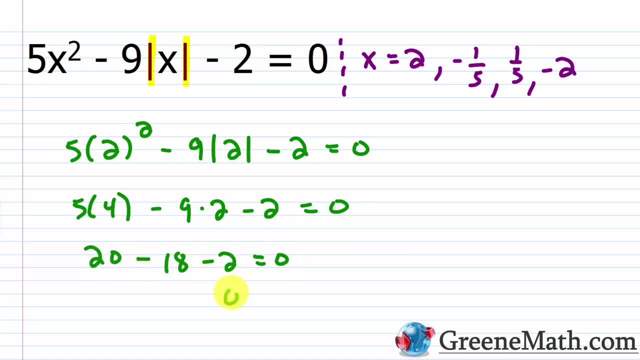 to work out right: 20 minus 18 is two. two minus two is zero. So you get zero equals zero. So this guy, Now let's work on negative 1, 5th now. So let's erase this and we'll do negative 1: 5th. So I'm. 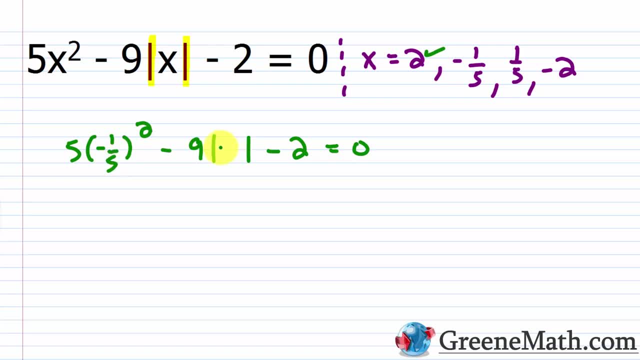 going to erase that and that I'm going to put negative 1- 5th in there. All right, So essentially, if I square negative 1- 5th, I would get 1- 25th. So we have five times that guy. then minus nine. 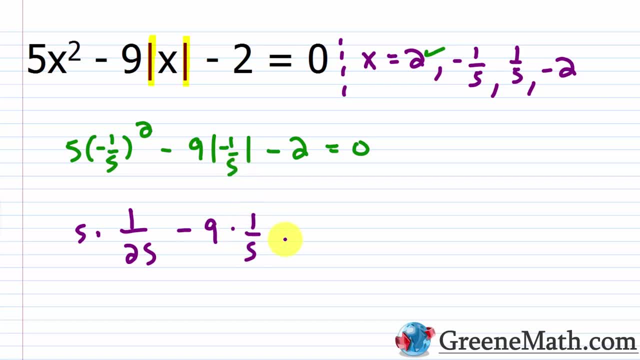 times The absolute value of negative 1 5th is 1 5th and then minus two, and this should equal zero. So this guy is going to cancel with this guy and give me a five. So you've got 1 5th minus. 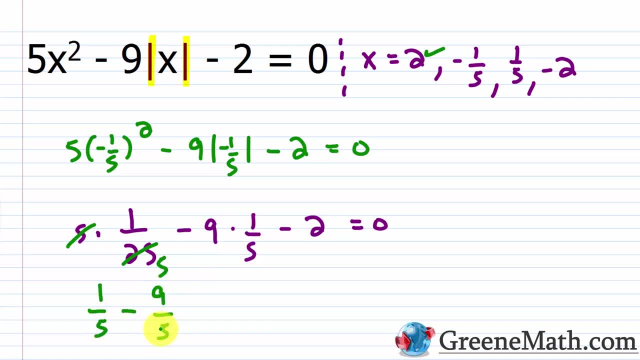 nine fifths. You can go ahead and do that real quick because they have a common denominator: One minus nine is negative eight, So that would be negative eight fifths. So you have negative eight fifths and then we're subtracting away two, So I can go ahead and write that with the. 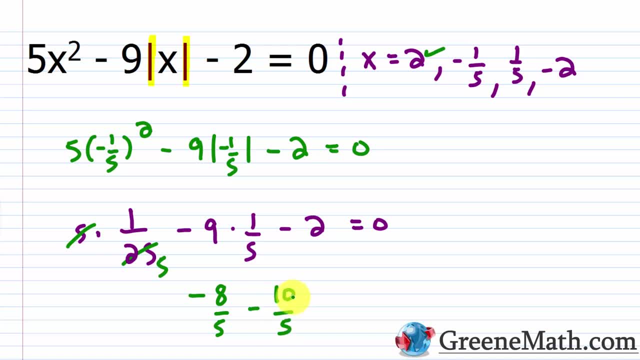 common denominator and say minus 10 over five. right, 10 over five is two and this should equal zero. And obviously it doesn't right. If we do this, it would be negative 18 fifths. Okay, Negative 18 fifths. So we're going to do that. So we're going to do that. So we're going to do that, So. 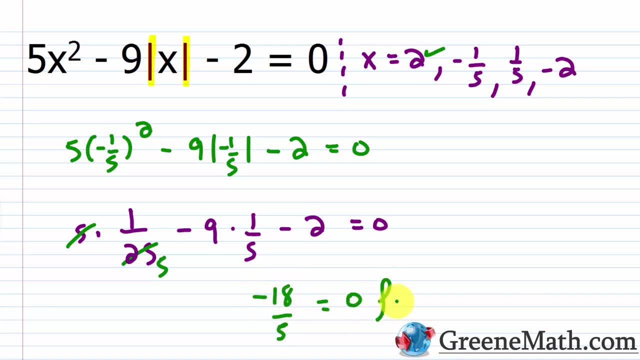 we're going to get 18 fifths, and that is not equal to zero. This is false, So we're going to reject that solution. Now I don't actually need to check 1- 5th, because I'm going to get the same. 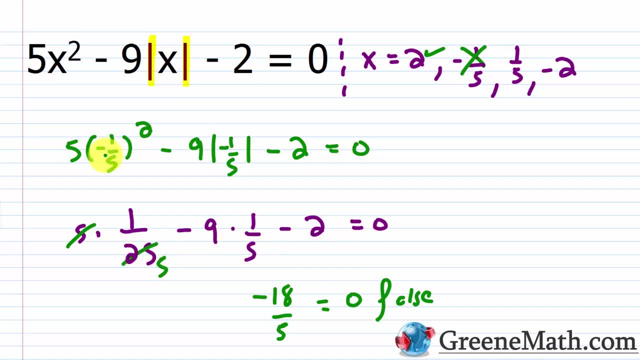 kind of result here. If I squared 1- 5th is the same as squaring negative 1 5th. In either case, I'm going to get 1- 25th. If I take the absolute value of 1, 5th is the same as taking the absolute. 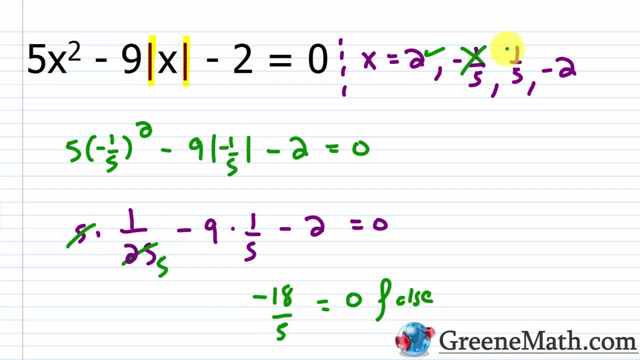 value of negative 1- 5th. So this would be the same and this would be the same, So you can go and reject that as well. Okay, So get rid of that. Then the other guy that you're going to have: 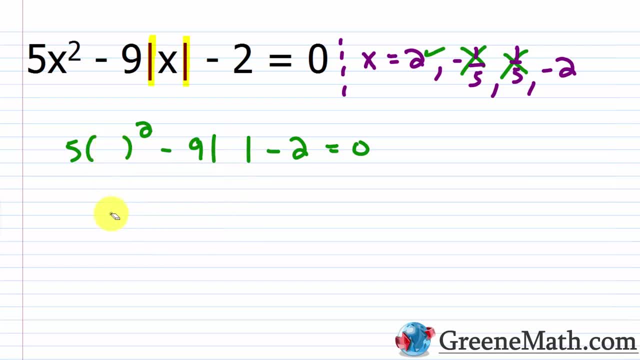 was negative 2.. So let's go ahead and check that. But again, you know that's going to work because 2 worked and you're going to end up with the same scenario, right? Because negative 2 squared or 2 squared each give you 4.. So in each case, you're going to have 20 there, because 5 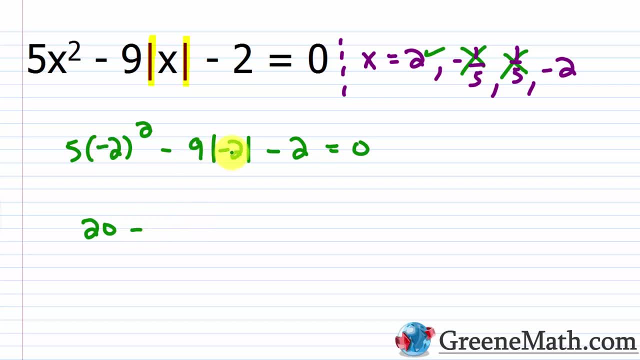 times 4 is 20.. Then you're subtracting away 9 times 2 in each case, because whether I put a negative 2 in there or positive 2, when I take the absolute value of that I get 2, right Either. 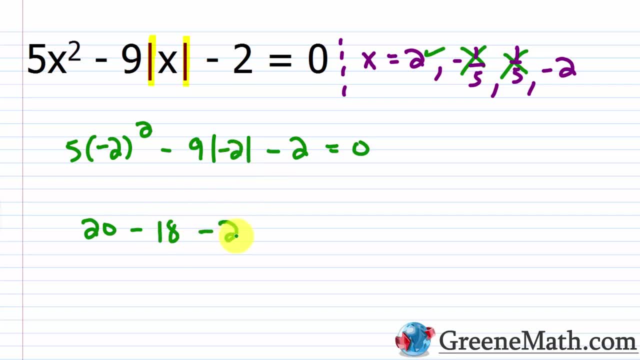 way. So 9 times 2 is 18.. And then you've got minus 2 and this equals 0. Again, 20 minus 18 is 2.. 2 minus 2 is 0. So you get 0 equals 0. So this does work out as well. 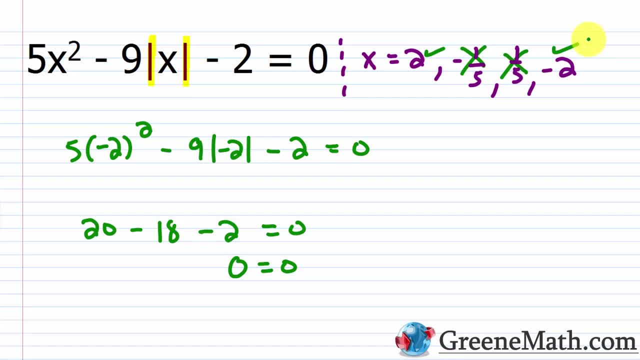 So this gave us two solutions: x equals 2 or x equals negative 2.. So I can just erase those, Just kind of tighten this down and say negative 2 there, And now let's think about doing this in alternative way. So for this method we're going to focus on using a substitution technique. 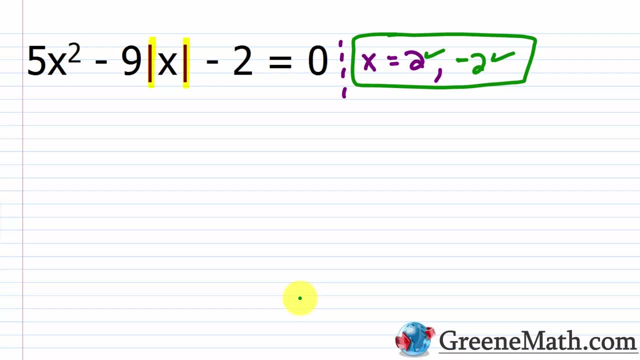 We use substitution to solve things earlier in the course, So it shouldn't be something new for you. Basically, what we're thinking about here is the fact that x squared is always nonnegative, and so is the absolute value of x squared, right? So if I think about x squared and I think about 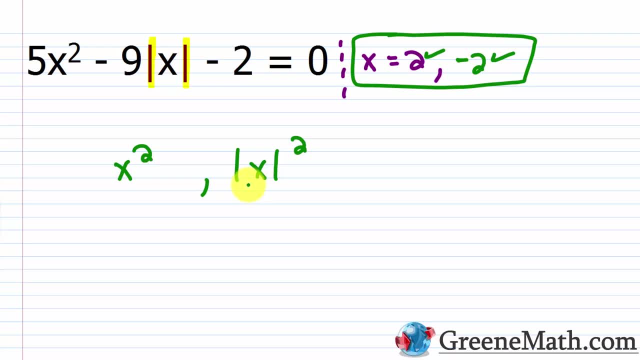 the absolute value of x being squared, this would produce the same thing, no matter what I plug in for x, right? If I plugged in, let's say, negative 3.. Let's say I plugged in a negative 3 in each case. Well, here, negative 3 squared is 9.. In here, negative 3, if I take the absolute value first. I get 3.. When I square that, negative 3 minus 3 equals 9.. I take the absolute value of x and get 9.. I take the absolute value of x plus minus 3.. I take the value of x and get 7 right there, And then, if I 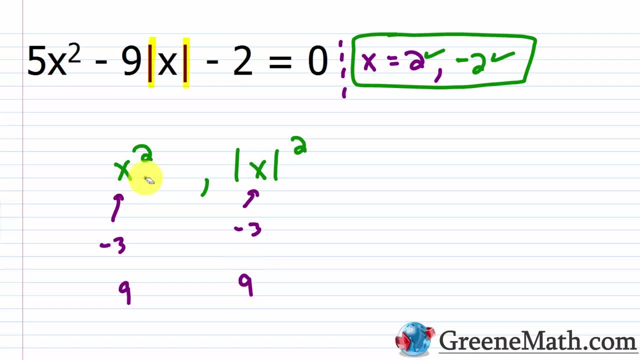 put my integration here, the absolute value gets small saved. Well, that's life. So if you want to do that for everything that, I get nine as well, right? So what I can do here is I can just rewrite this And I can say: 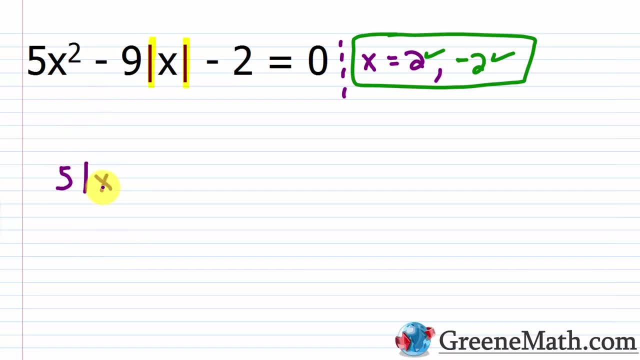 that we're going to have five times the absolute value of x- that's squared- then minus nine times the absolute value of x, then minus two, and this equals zero. Okay, so now I have the absolute value of x here and I have the absolute value of x here, Okay. so what I'm going to do is just: 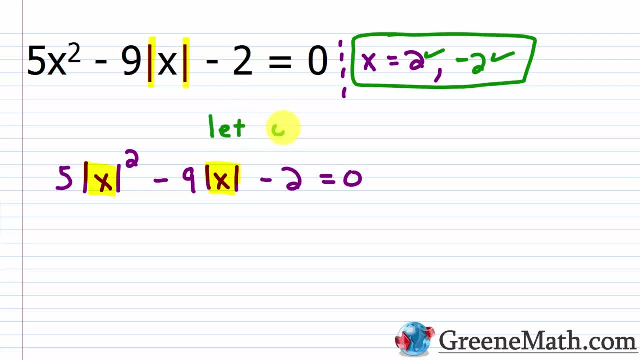 make a little substitution. So I'm going to let u be equal to the absolute value of x. okay, So now I'm going to replace the absolute value of x in each case with u, So I'm going to have that five u squared minus nine u minus two is equal to zero. So this is something we can again solve using. 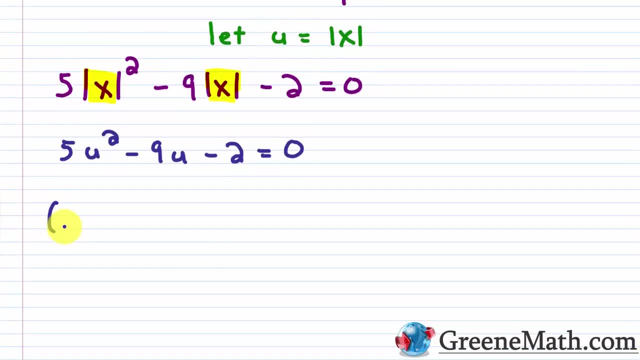 factoring. Let me kind of scroll down for a minute. So I'm going to put a five u here and a u here. this equals zero And of course I need my outer and my inner to sum to negative nine u and my final to be 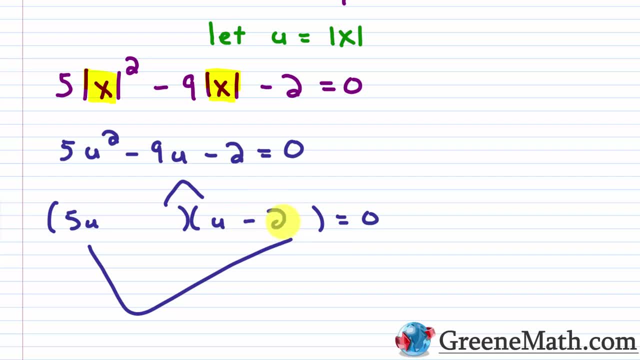 negative two. Okay, so we know we're going to do that with a negative two here and a positive one here. We saw that earlier. Okay, so we know that five u times negative two would be negative 10 u and that one times u would be plus u. So this gives me my negative nine u And, of course, 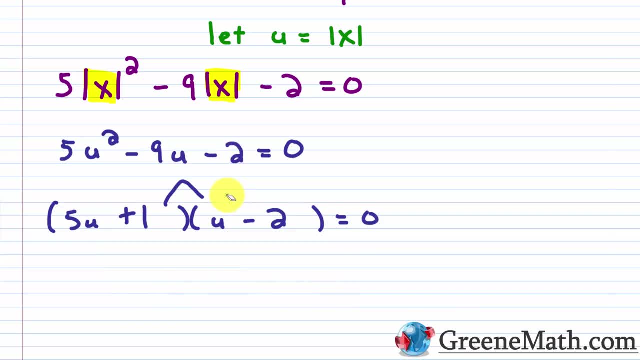 one times negative two is negative two. Okay, so let's erase this And let's kind of solve this real fast. So I would set five? u plus one equal to zero, And then I'm going to put a negative two zero subtract one away from each side of the equation. you get five? u is equal to negative one. 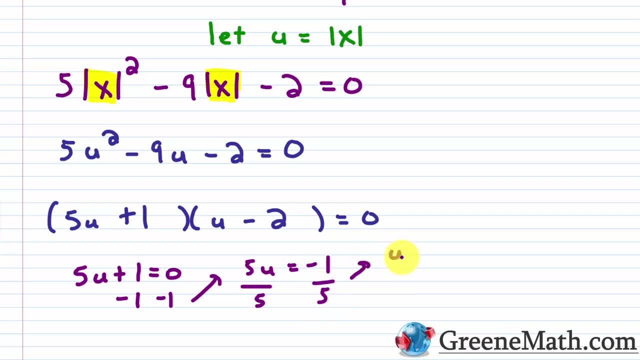 we're going to divide both sides by five And we're going to get that u is equal to negative one fifth- Okay, so let me write that over here: u is equal to negative one fifth- Okay, so let me erase this. I don't need that anymore. The other guy's really easy. you can solve that mentally. 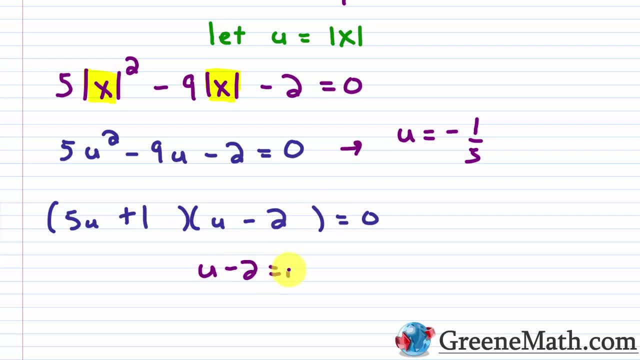 you have: u minus two equals zero. So u minus two equals zero. add two to both sides of the equation and we get u is equal to two. Okay, so let's put a two there. So you might be thinking you didn't get all the same solutions that you got. 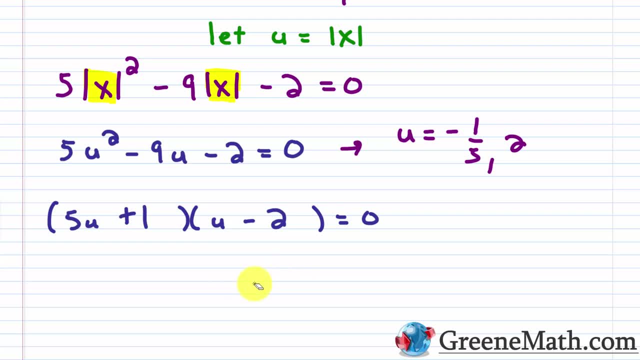 using the previous method. Well, we did. we just have to go back and substitute again. So let me erase all of this. we don't really need it anymore. Okay, we're just going to scroll up. we're going to think about what u means. So I told you that.